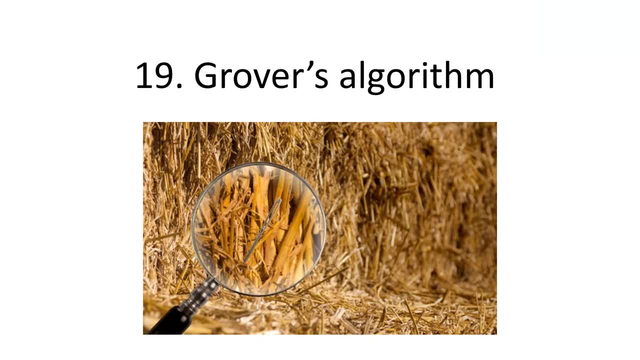 And also, like: is it possible for us to have like some kind of like the exam from the past years? Okay, all right, sure, yeah, I'll upload something like that, yeah, for one of the past years. I think it should be kind of similar material, so yeah, but I mean, I think you've seen, you know already. 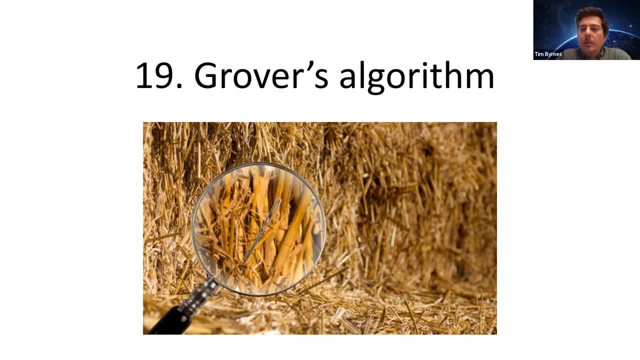 basically what the exam will be, I mean just based on the midterm. it will be similar style to that, So you can just like, just want to practice for like the kind of the kind of questions that we studied, like after the midterm. Sure, of course, yeah, okay, all right, yeah, so this Grover's algorithm is. 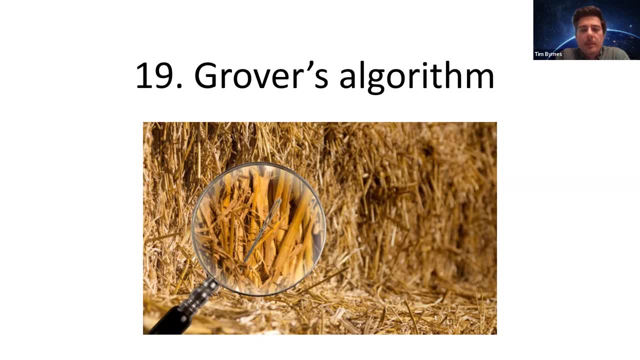 like I said, one of the famous quantum algorithms that are sort of known, You know, there's not, you know, unlike sort of classical computer algorithms, there's not, like you know, sort of so many algorithms that are, you know, useful. that actually shows you a speed up over classical computers. 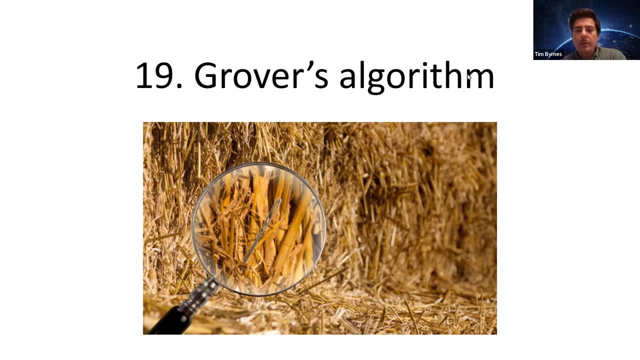 But Grover's algorithm is one of them and it's very useful. So this picture that we've got here as well, I'll try to see this- is, like the, the basic task of Grover's algorithm, which is to kind of find a needle in a haystack. So this English expression, needle in the haystack. 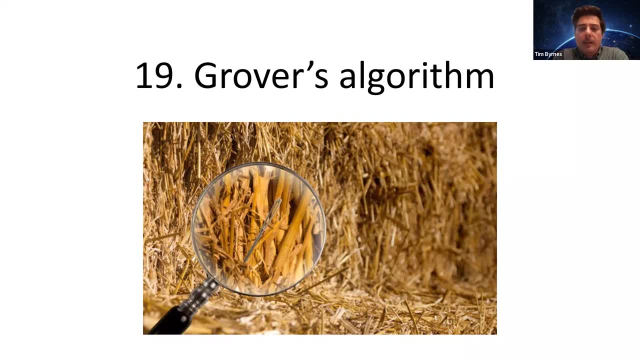 you know, it's like trying to find something which is very hard because of course the haystack is pretty big and needle is very small and also needle kind of looks like hay. so it's, you know, very difficult to find. So finding the needle in the haystack is basically the aim of Grover's. 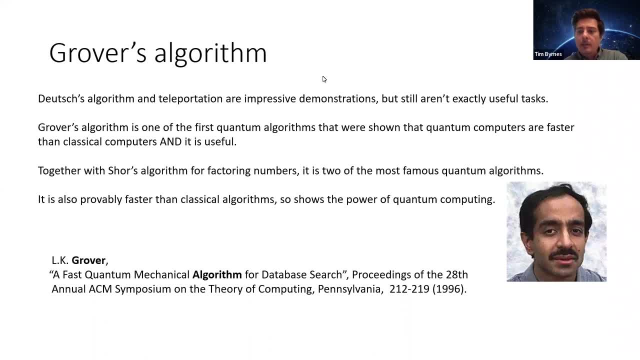 algorithm. So just to give you a bit more background on Grover's algorithm, well, this is Mr Grover, here's the Indian guy and- and this was, as I said, one of the first famous quantum algorithms- Deutsch's algorithm is like perhaps the first quantum algorithm that shows a quantum speed up. 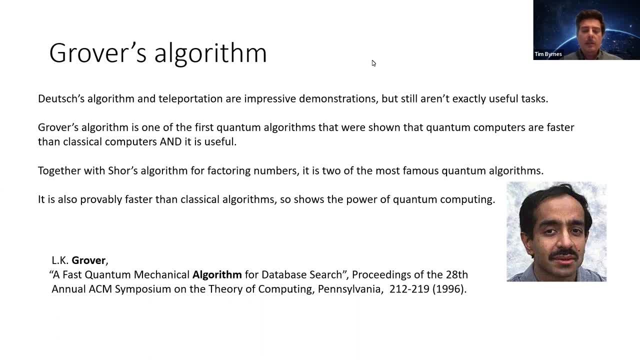 but as we've kind of discussed, you know they're not particularly useful algorithms. You can't really use Deutsch's algorithm for anything, except for a kind of a demonstration to show that it's possible to actually do something faster with a quantum computer. but Grover's algorithm is actually something that is potentially extremely useful. 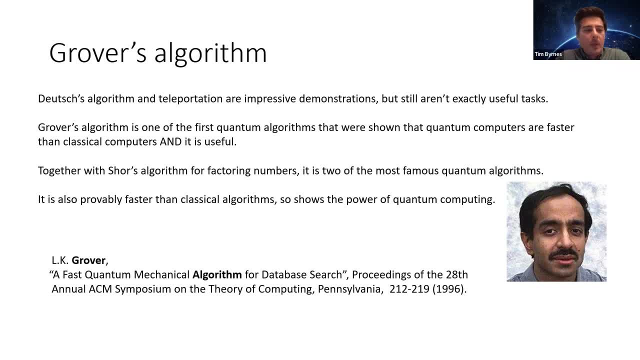 So it's, and it shows a quantum speed up. So I would say that maybe, if you were to name the two most famous quantum algorithm, they they would be: Grover's algorithm would be one of them, And perhaps the the most famous quantum algorithm is Shaw's algorithm. 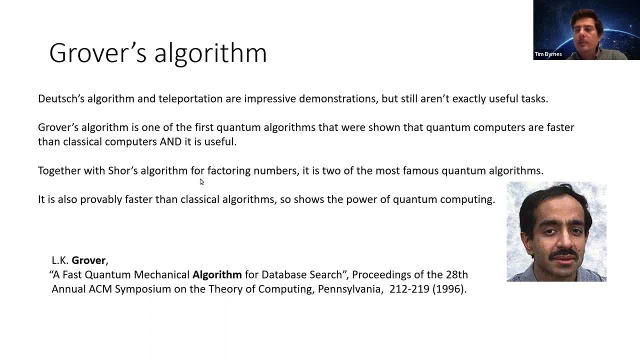 and I don't think we're not really going to have the time to do this one, because Shaw's algorithm is a little bit more complicated than than some of these other algorithms. but the task that Shaw's algorithm achieves is to find factors of a number. So if it's like you're given the number 21, 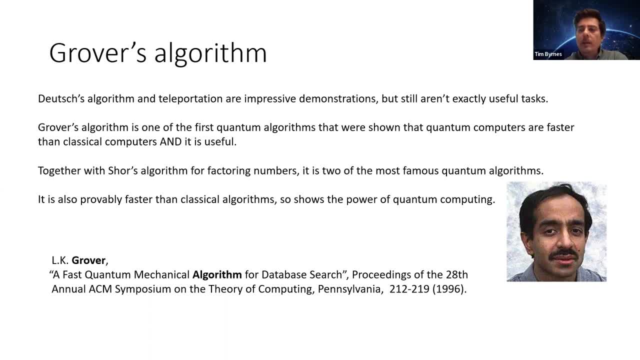 the algorithm would be able to find that, you know, the factors of 21 are equal to 7 times 3. So it gives is the factors, and it can do this exponentially faster than the best known classical algorithm. So it's quite a spectacular example of a quantum algorithm. So Grover's algorithm. 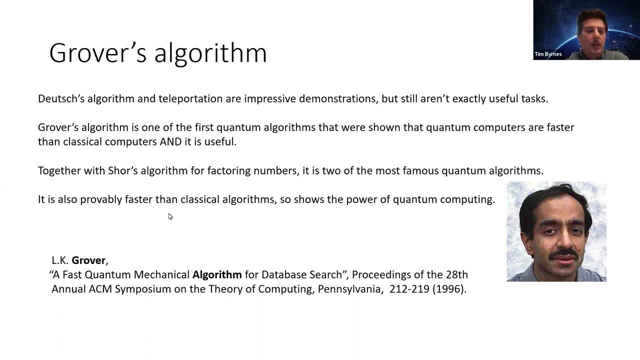 as I'll show you, is a kind of a search algorithm and you it's actually. it's also provably faster. so this Shaw's algorithm is, like, exponentially faster than the best known classical algorithm. You know there might be a faster way to factor numbers like a classical algorithm. that is actually faster than you know something. 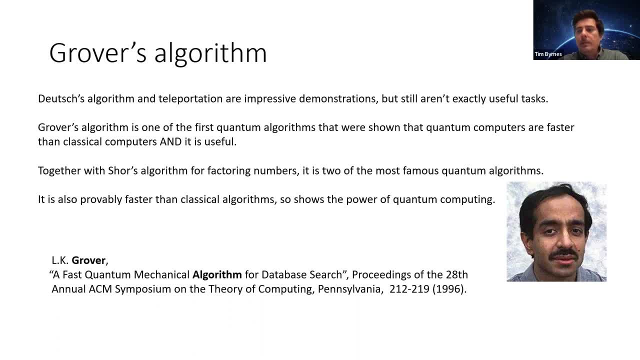 it takes exponential in time, you know, but it's just that the best known one actually, uh exponent, there's an exponential difference, whereas with gerber's allen, actually we know for sure that the quantum algorithm is faster than the classical. okay, those uh originally shown in this paper, 1996.. so what is it? so this is the kind of problem that we're talking about. 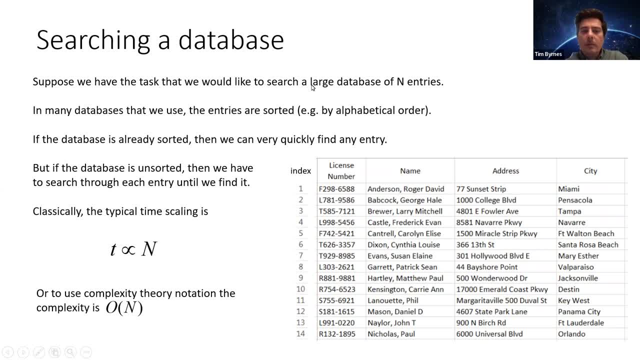 so suppose we have the tasks, that we want to search a large database and it has like n entries, okay, so an example would be: like i've got just down here, uh, here i've got you know sort of a database. uh, it's got you know names of people and their addresses. 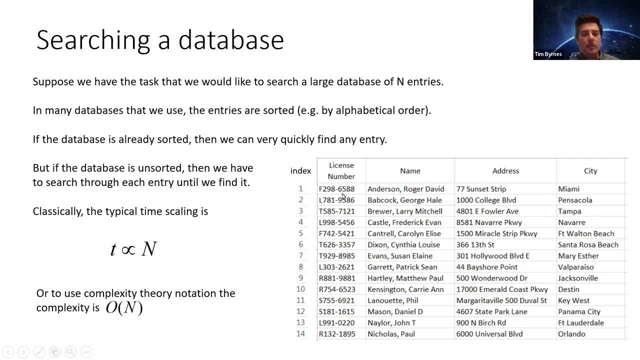 and then the city that they live in, the license number of their car- oh sorry, maybe their driver's license here, and well, they're just numbered from one, you know one one, to some number 14 here and um, what we want to do is to kind of search through this database. 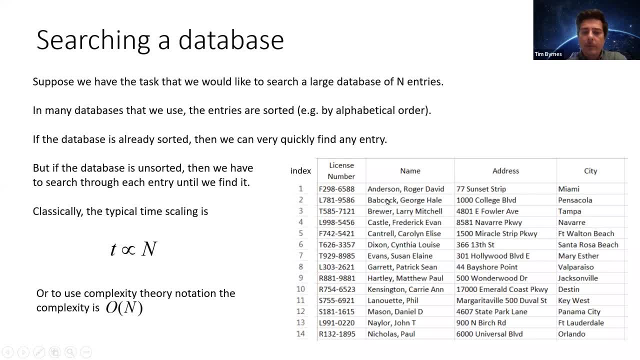 so that's the kind of task and, uh, if we were trying to search by name, of course, uh, this is, uh, you know, not such a hard problem. so if i were to say, you know, okay, i want to find the guy that's like evans right now. um, of course, these names are ordered alphabetically, and so, even if this- 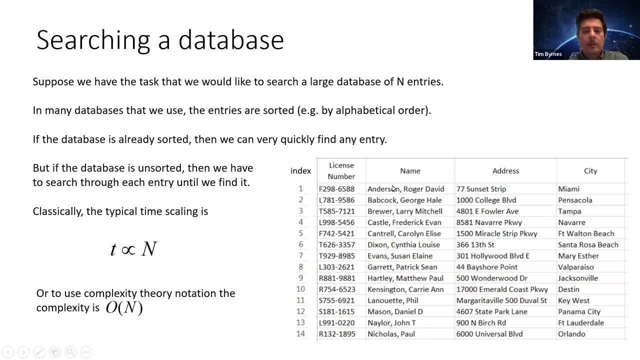 database contains, like you know, a billion names or something like that. uh, it wouldn't take you very long to find the name because, of course, uh, you know, you can just search for it alphabetically. so we have some convention, you know, alphabetical order. and actually, even though there's 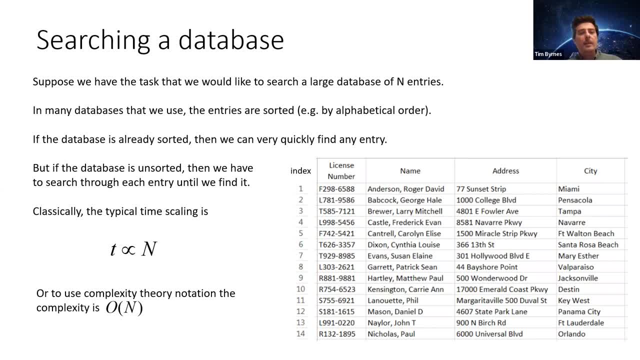 a huge number of names in there. you can quickly find it because you know it's all ordered right and so you can easily find, uh, each entry. but uh, if the database isn't sorted, then it's not as easy to find right. so if i were to instead say okay, 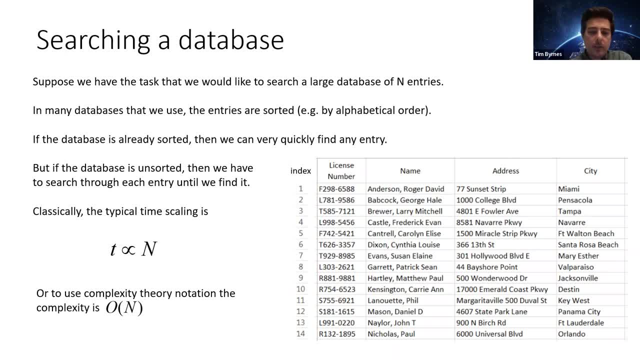 you know, find me the entry uh, where the license number is. you know uh ends like, say, in the forward four digits of um. you know, zero two to zero, uh, because these license numbers are not ordered basically, well, not basically, you know, actually what you have to do is to just go through and 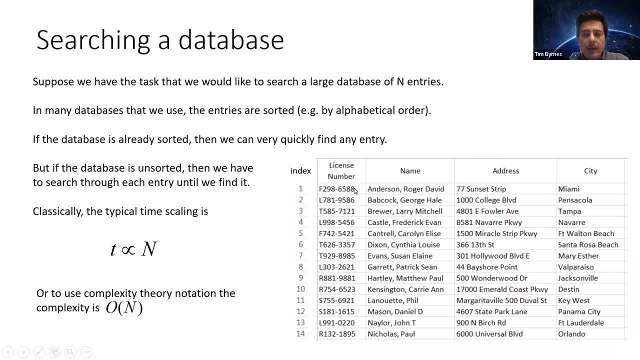 check each one, because there's no ordering or anything like that. uh, you have to look at each number. so you're looking for zero, two to zero. so it's like no, no, no, no, and you go: okay, this one number, thirteen, um, you basically have to look through. 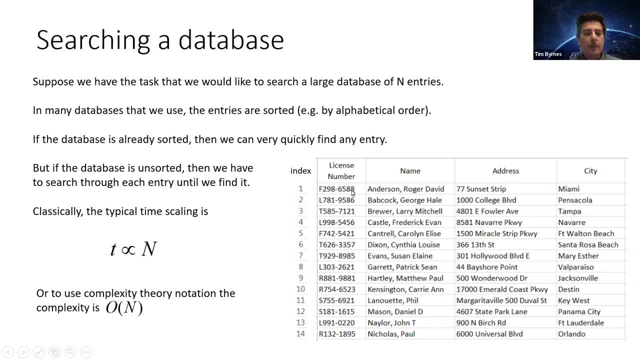 uh, the whole database and, okay, you might get lucky, it might be in the first, first half, but well, in this case it was in the second to last. so you ended up looking through, uh, almost an entire database before you found it, and there's not really any other way of doing it, like in an 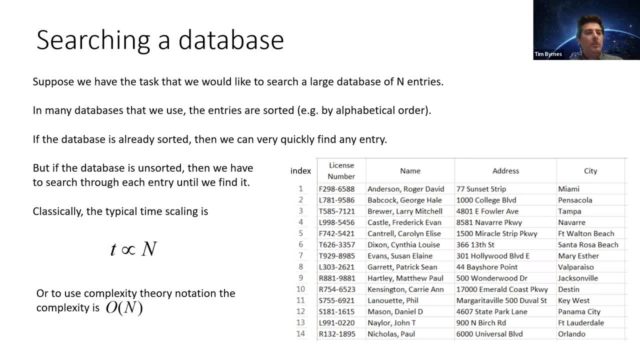 unsorted database there's. there's just no strategy that you can use because you know the ordering of all these things are kind of random and so you know, if you were just to do this randomly, this had uh n entries on average, it's going to take well n over two, right sometimes. 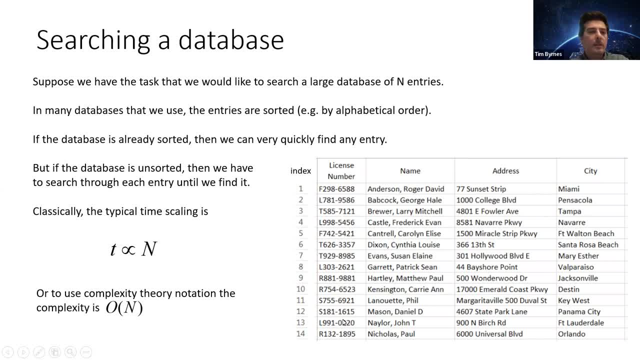 you get lucky. sometimes it's uh, you know you'd be unlucky and then you know on average it might be something like. you know, we normally don't really care about the uh, this kind of n over two, so we the important thing is that we say that it scales with n, which is the number of database entries. 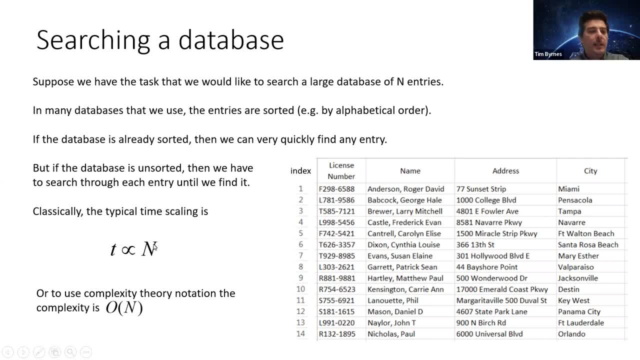 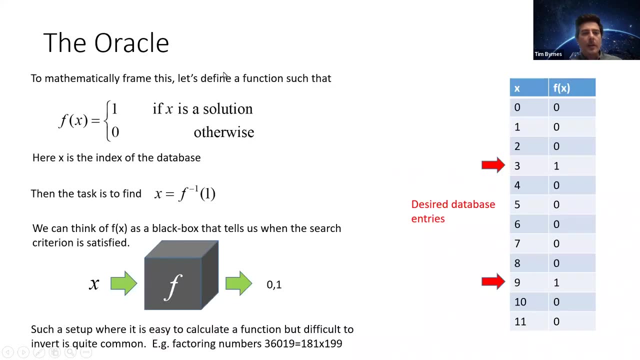 okay, so, okay. so, forget about the proportionality factor, just say how it scales with it. so in computer science kind of way of saying, it would be that the complexity of this is: uh, order n, okay, so, um, uh, the way that we're gonna, uh, so let's kind of abstractify this problem a little bit. so 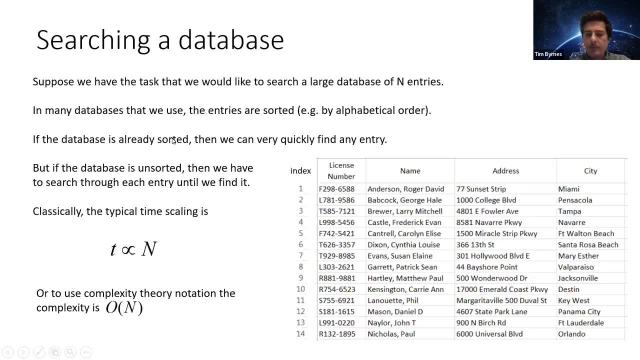 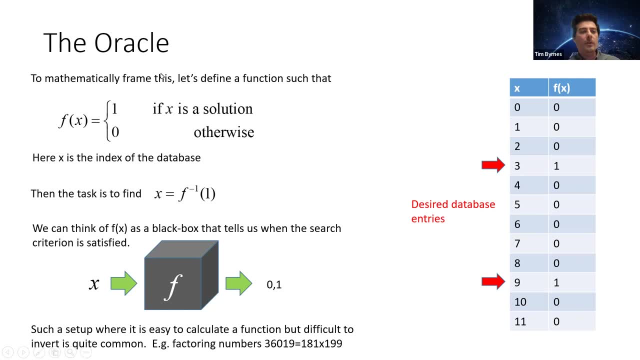 let's say that the uh, instead of having this kind of you know database that we have here, um, we're gonna work instead with, uh, what's called the oracle. so the oracle. we already uh heard something like this in the previous slides. uh kind of, for example, in the deutsch's algorithm, we also 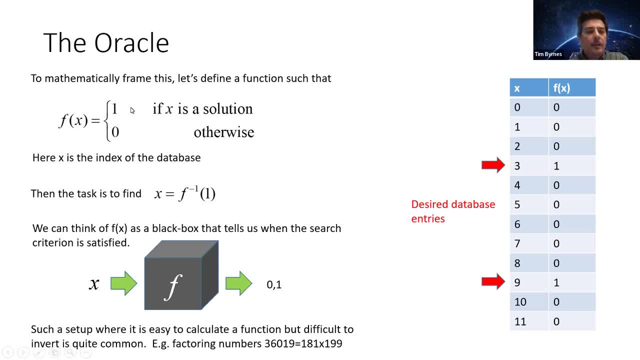 talked about an oracle. um, so basically the oracle is, you know, instead of having this kind of database of numbers and names and stuff, we just let's just have a function that you have, um, you know, ones and zeros as the output. uh, x is the index. okay, so say: uh, here we've got the index number. 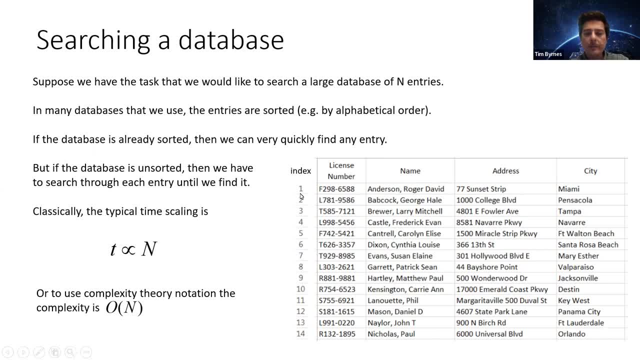 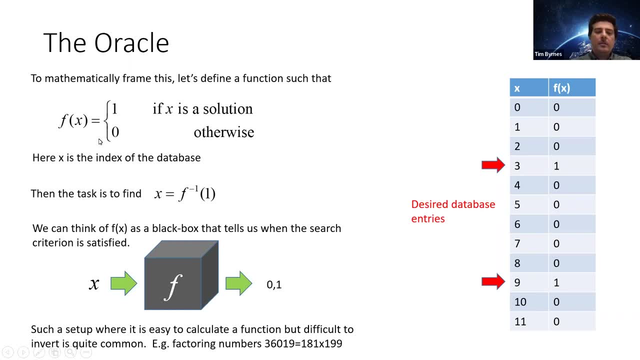 so we're just going to label each of these entries by a number like this, and then, uh, f of x is basically something that tells you whether that's the solution, or you know, that's basically just a marker, just to say whether this is the thing that you're looking for or it's not the thing that you okay, so, uh, so, for example, 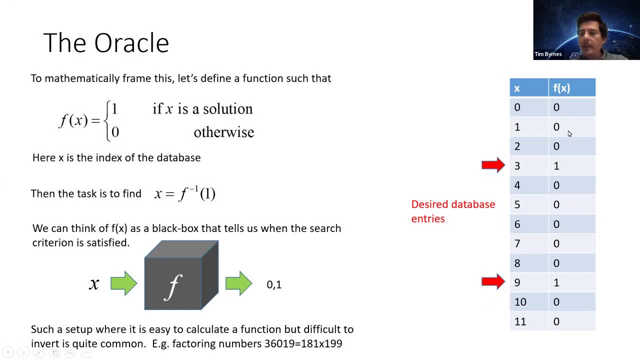 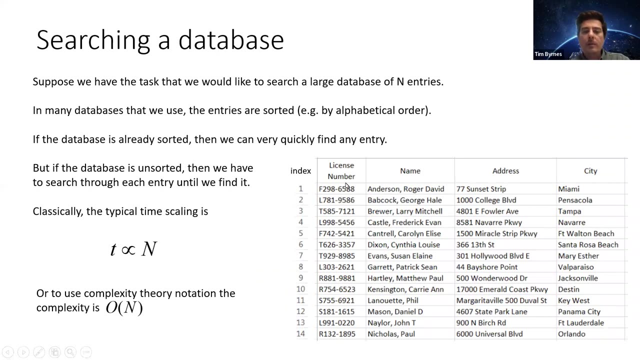 over here, um, maybe this uh function here could be something like um, and you know, it totally depends on the question, of course. so here, uh, it might be something like um, i want to find all the people where you know say the last digit is uh, six or something like that. so in that case, 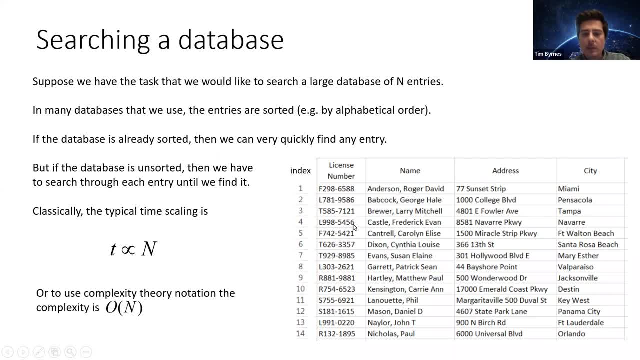 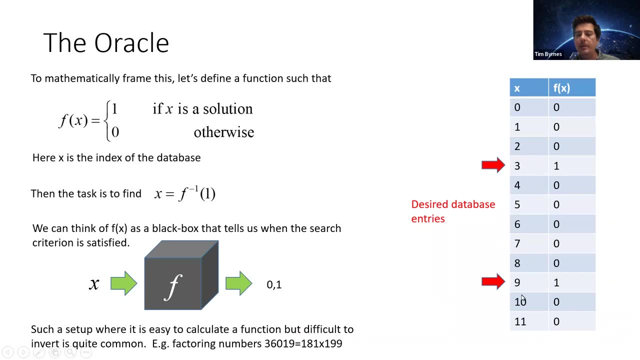 you look at the last digit, then here here's one with six, here's another one with six, and then all the other ones don't have six. so it's number two and four. um are the ones that we're going to be looking for. so, in this case, um, okay, uh, for this example, number three and number nine are the ones. 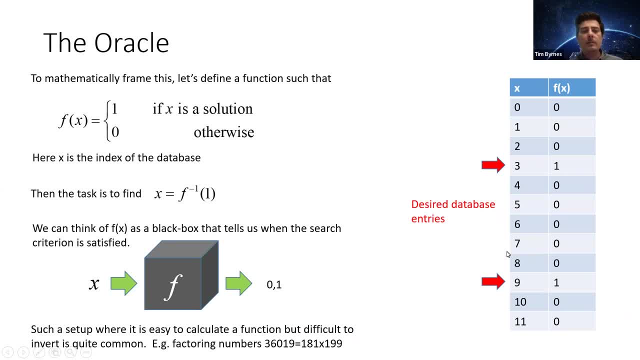 that we're looking for in, you know, whatever it is, the thing that we're, you know, kind of trying to, trying to search, search within. so, basically, f of x is just the thing you know points out solution, and then, uh, what we're trying to do here is, of course, find which ones are the solutions, right? so 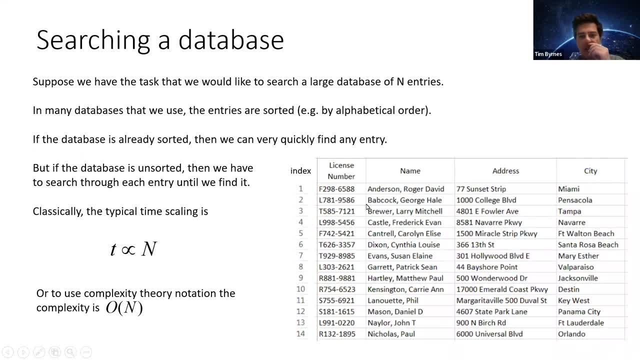 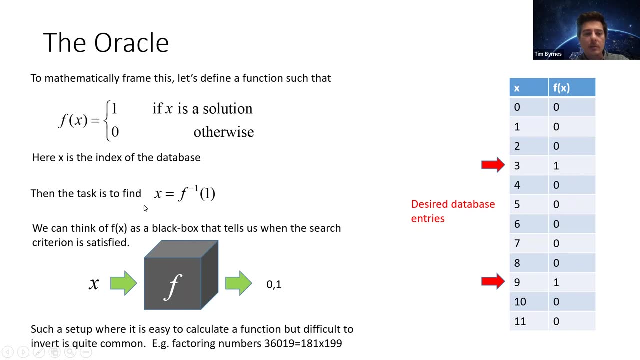 you know, the aim here is like: okay to you know, you want to find, okay, which is, which are the people with? six is the last digit in the license number, so the answer is two and four, okay, so in this case, basically, what we're trying to do here is to uh, find this, uh, the solution of this. so basically, 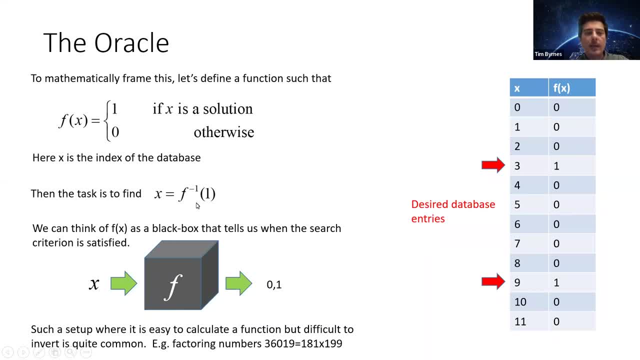 uh, f inverse one, which are the solution cases. we're trying to find all the cases where x, well, f of inverse is one, okay. so, um, we can treat this, you know, think of the oracle again- as some black box. uh, we don't have to really think about, like, what's inside the black box, even though, well, 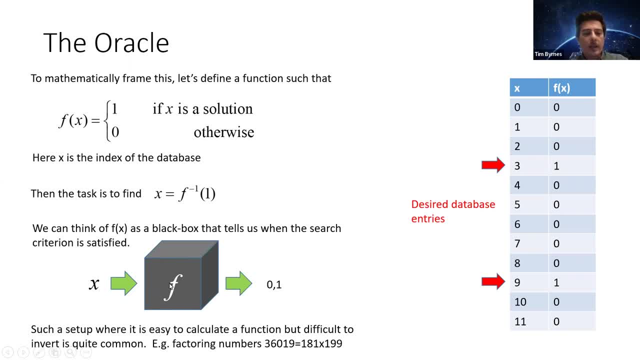 you know, you could always think of a circuit that does this and um, so, uh, usually what? what? uh? the situation that you have here is that, um, finding this inverse is kind of a pretty hard, hard problem. okay, so it's easy enough to just plug in x and then find f of x. 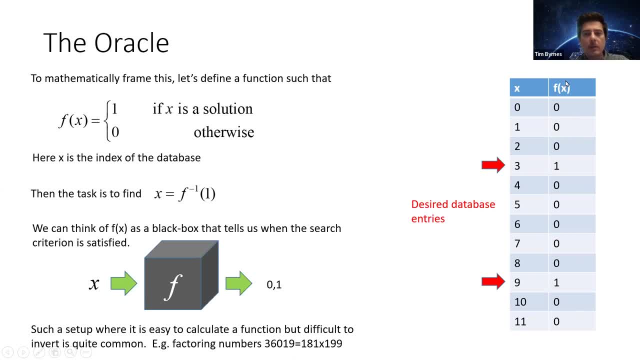 but if you say which ones of of the f, of x's are one, well, uh, basically this is again a search problem, because you know, the only way that you can really find this in general is to look through all these cases and then find the ones where the answer is one: okay, so you have to look through. 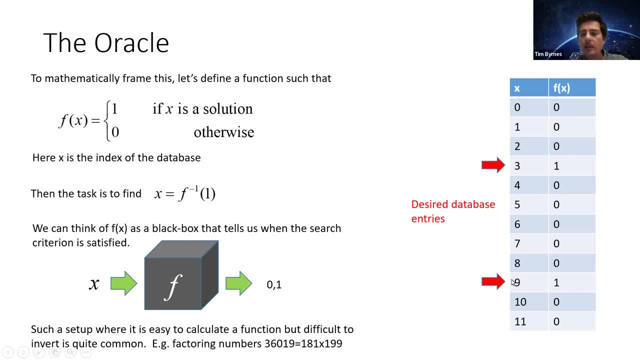 all these ones, and then you say, okay, fine, three and nine satisfied. you know this equation here. so, um, usually this kind of oracle, it's sort of easy to go forwards, but then it's kind of hard to go back. so this is a kind of a pretty common setup and in fact this is often what's. 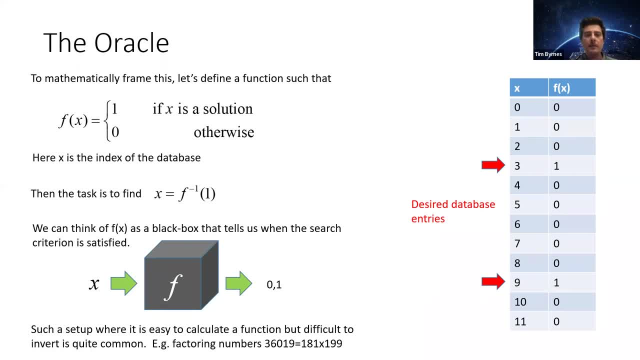 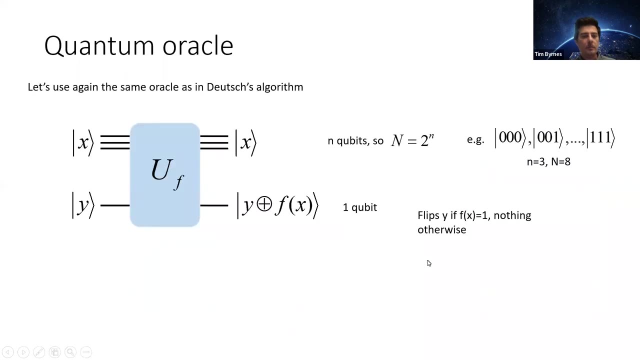 used in uh, cryptography and things like this, because, um, you have these sort of one-way functions where it's easy to calculate one way but hard to go the other way. okay, so we're going to work with this kind of oracle function now, and what we're going to do is we're going to allow this oracle to be like a 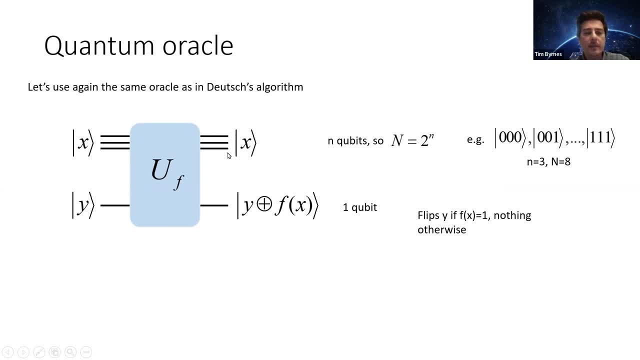 you know quantum oracle, okay, so that basically means that we're going to allow it so that the input of the oracle can be in like a superposition state. so you've got, this is the input state. so we're going to have basically, basically the same kind of setup. 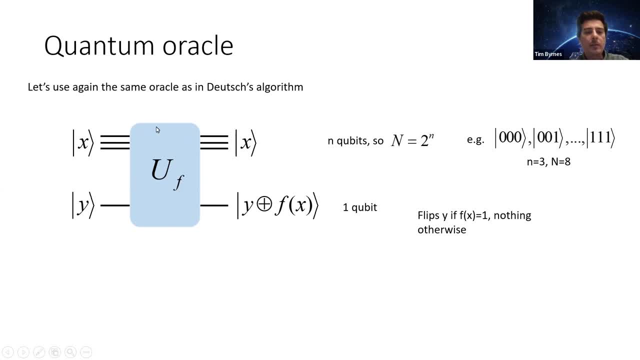 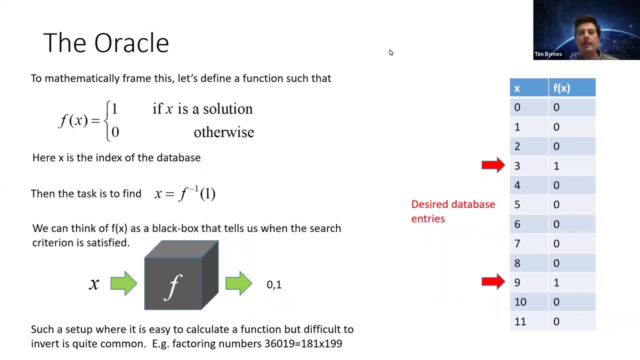 as we already saw in Deutsch's algorithm, And so remember, in Deutsch's algorithm we couldn't just have, like a Oracle that just directly does something like this, where you have X and then you have the Oracle which contains the function X, And we couldn't do something like this. 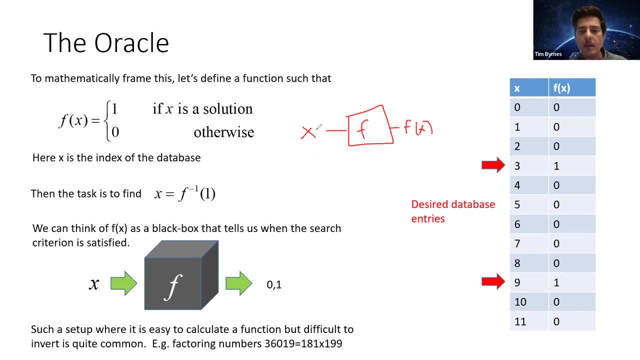 basically because this was not a unitary process, right? So imagine if you get the value zero over here- well, there's lots and lots of cases that actually give zero right- And then if you found the output to be in, well, I should really say zero state. 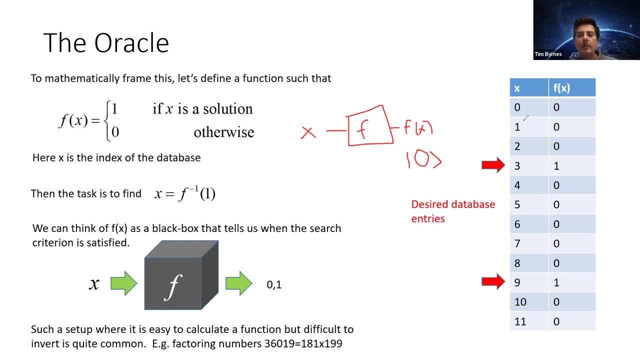 So if you found the output to be in zero state, there's no way that you could figure out in general which one was the input state. So this way is basically: it's not an invertible function, So we can't implement that with quantum mechanics, okay. 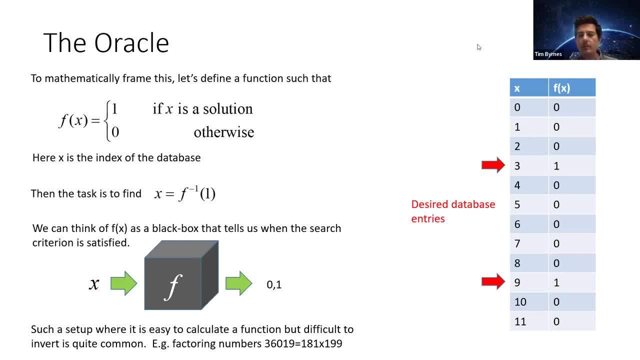 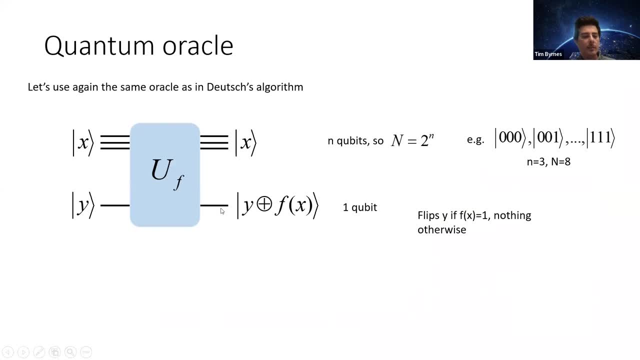 So that's why we eventually went with this type of circuit on the next page, because this is an invertible kind of way implementing this Oracle. So we, instead of having the output as just f of X, we have the output as just adding modular to f of X. 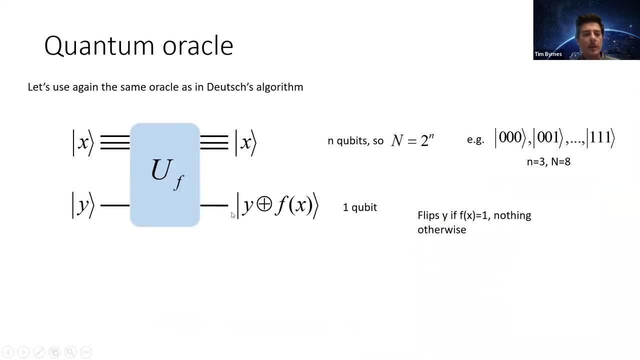 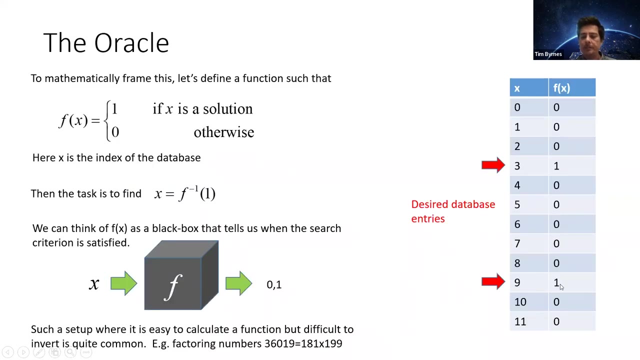 And where, in this case, f of X is like this function And then we just add that into the Y, okay, And so basically, what this is gonna do, it's gonna flip if f of X is one which is like one of these solutions here. 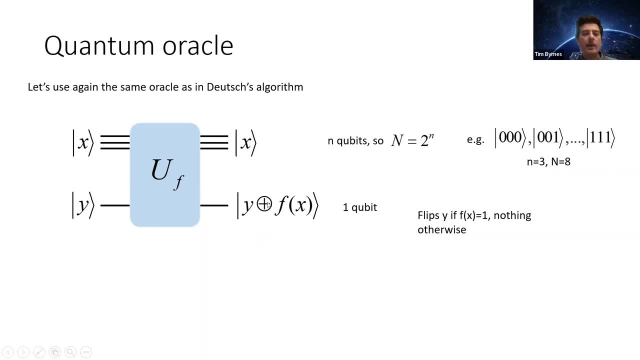 it's gonna flip the output, the output of this one, So it's gonna be Y plus one, then modular two. So if this Y was one, then if this was one, then if f of X is one, then this would become zero. 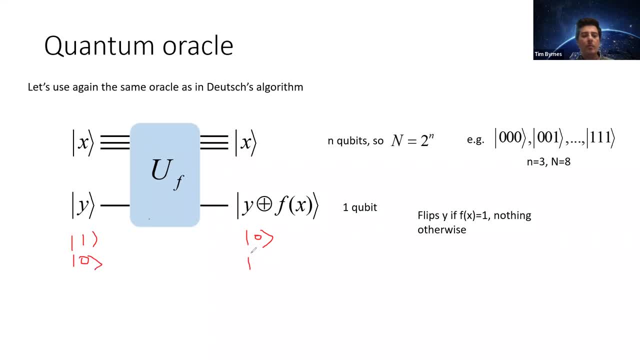 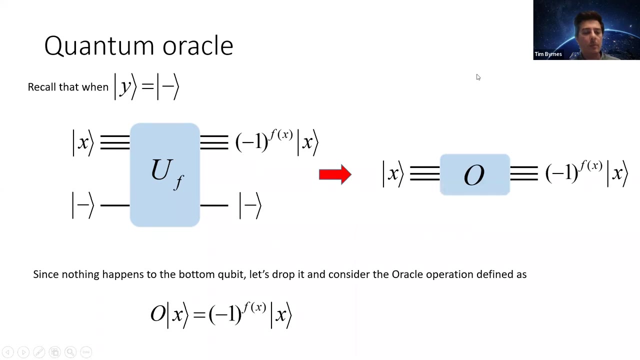 And if Y was zero, then Y plus one would be one. So basically same setup as Deutsch's algorithm. If you remember how that is okay. So that's how we're gonna implement the quantum version And then remember that also in the Deutsch's algorithm. 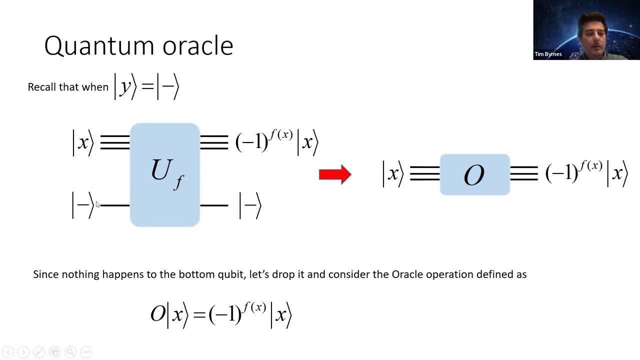 what we did was eventually we prepared this input state here to be a minus sign, okay. And then, if you just recall what happened with Deutsch's algorithm, what basically that eventually does is, if you start with this state X, then it will output the state again X. 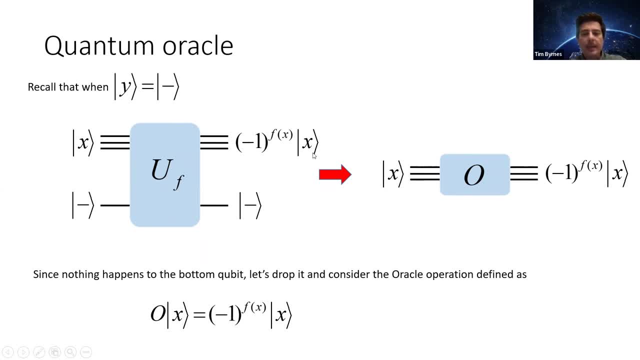 but then with a minus one phase here, And so actually, because nothing really happens to this lower part of the circuit, we can just kind of omit it or just well, yeah, just don't show it in the notation. And so what we're gonna actually use is something like: 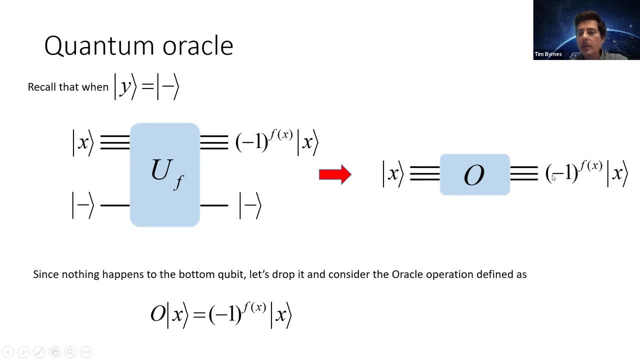 this where basically X becomes a minus one to the power of F, of X, And that's basically what we're gonna consider the oracle. Now I think I said this for the Deutsch's algorithm as well, but to me like this whole thing with the circuit. 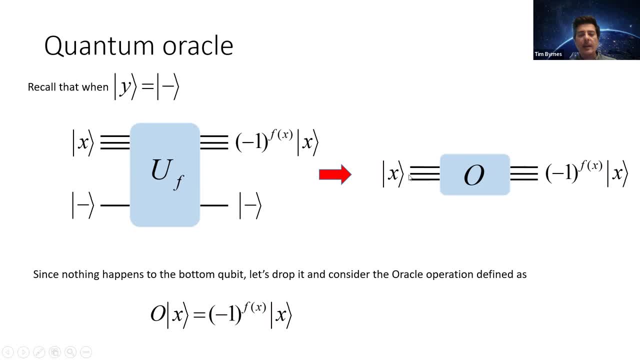 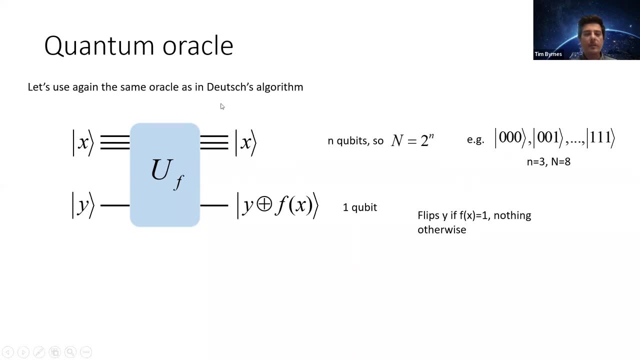 and putting the minus state in and all this. actually it's sort of a historical thing. So, if you like, if you don't, if you find this, this whole thing with the UF there, F and the, this, putting the minus state in. 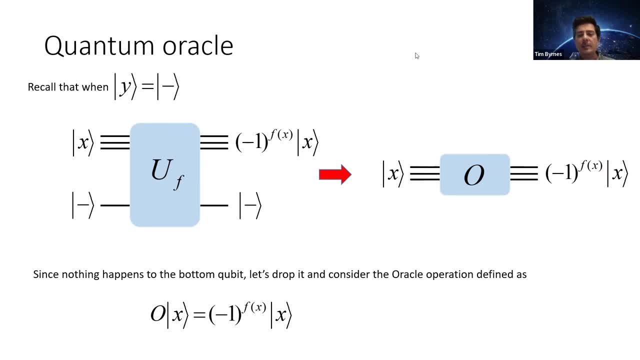 if you find that whole confusing thing confusing. actually, instead, what you can- I think it's just basically the same thing- is to just say that okay, we're gonna implement the oracle using this kind of formulation, where basically the input state is X. 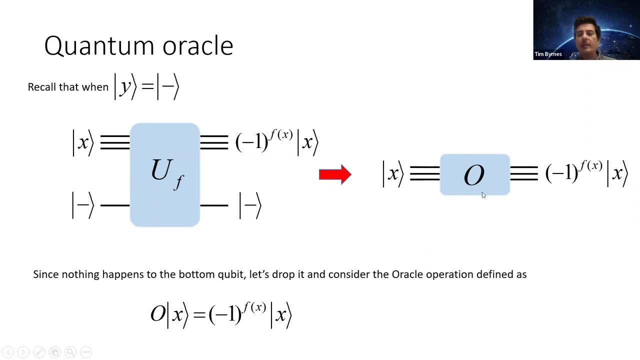 and then the output state is minus one to the F of X, And if you just say that that's gonna be my definition of the oracle, well, this is a perfectly unitary transform, as you can see here, because if you start with this state here, 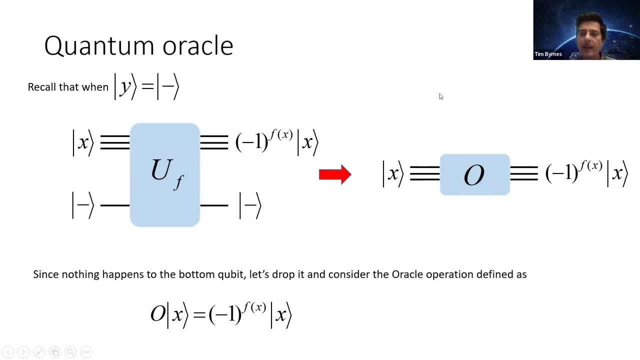 you can easily just apply this one twice and then go back to the initial state. So this is perfectly unitary transform. So if you just say that, okay, that's my oracle and that's the end of the story and that's how I implemented it. 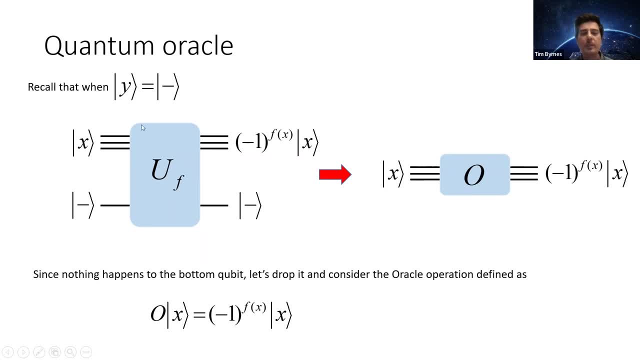 then you don't have to worry about all this, this kind of stuff which happened, which I consider a sort of a historical, historical origins of this thing. You can immediately jump to this if you prefer that explanation. So long story short. basically, we're gonna implement the oracle. 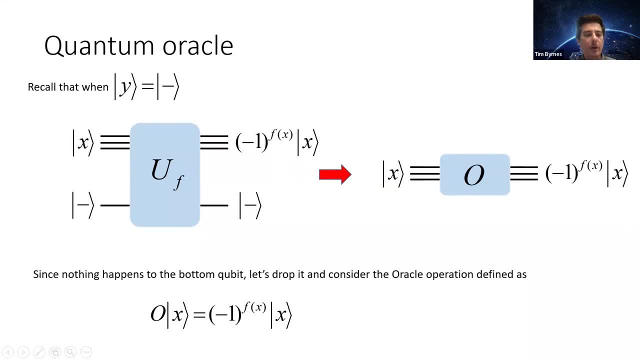 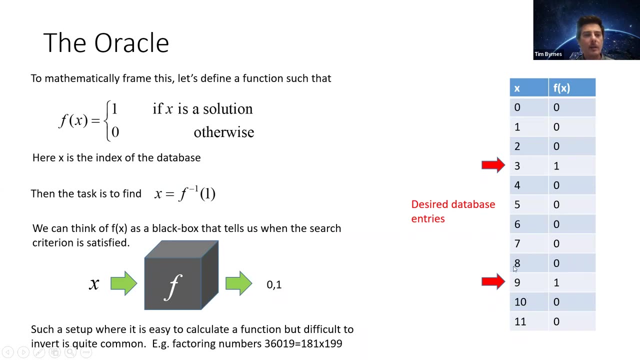 according to this kind of operator. So we have O as an operator here- gets applied to X, which is, again, it's the state form of basically all these database entries. So it's just the index of all the different cases. 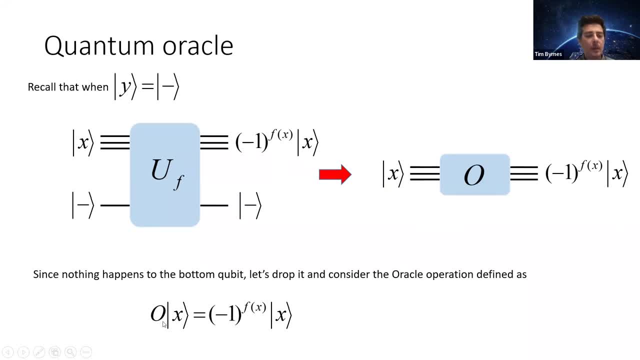 And basically, when the oracle gets applied to the state X, it has a plus or minus one phase, And so it has a plus one phase if it's not a solution, and then it has a minus one phase if it is a solution. Okay, 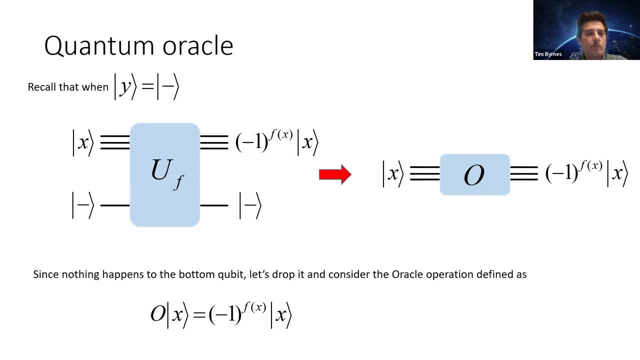 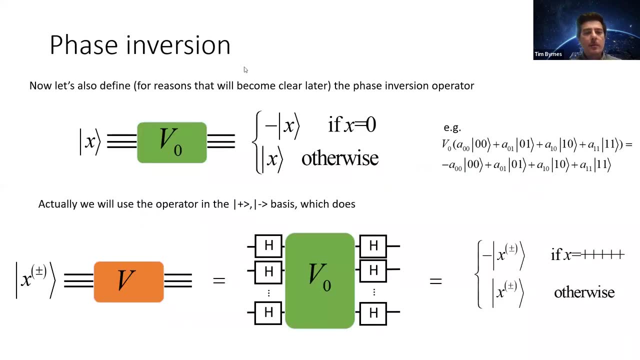 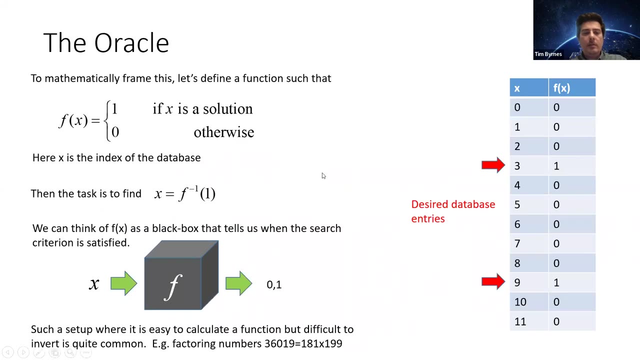 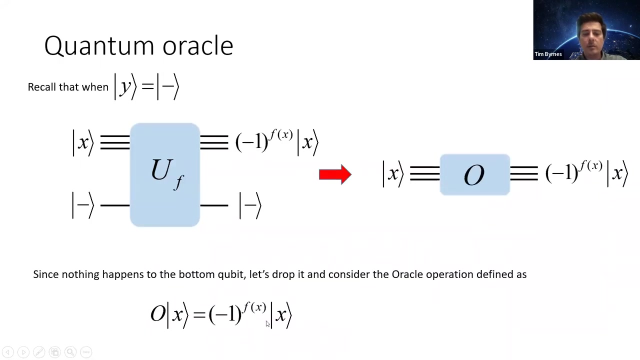 Does that make sense? Okay, Oops, So all right. So that's the oracle. Basically, we're gonna encode this box here as something that puts a minus one phase on the state. Now, what we're gonna actually also need is: 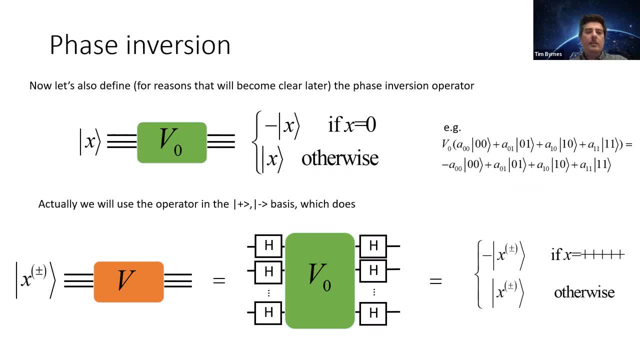 is another very similar type of operator, And this thing doesn't have a really good name, but I'm gonna call it the phase inversion operator. Okay, And it does just about the same thing. In fact, it's even simpler than the oracle. 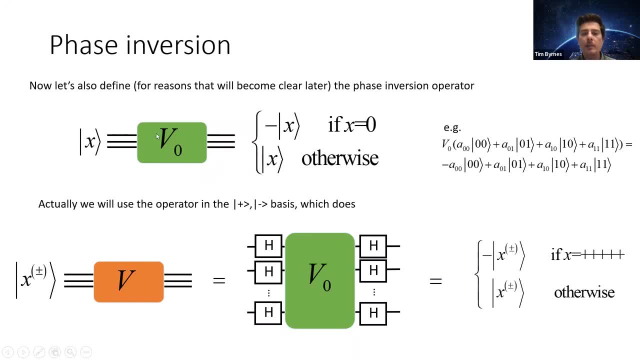 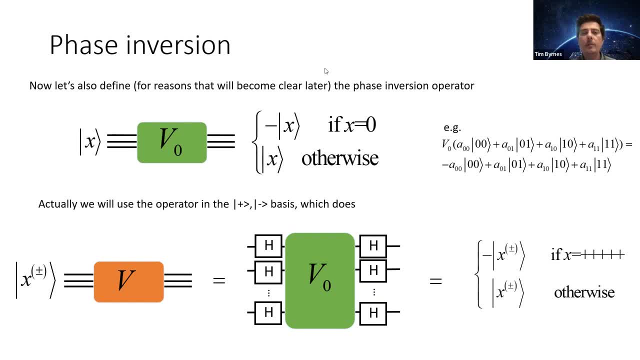 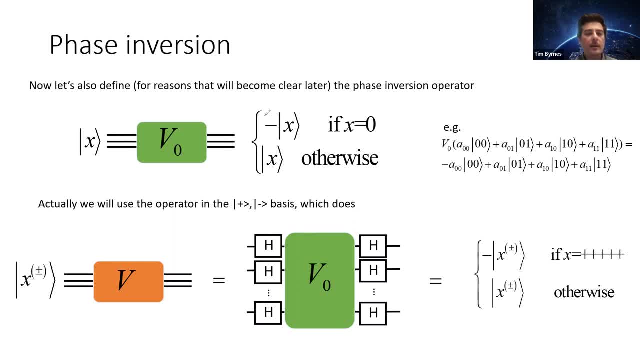 what I sort of mean by that. and notice I've got like multiple lines here. So for example, in this three qubit case, when I say X, what I actually mean is like the binary form of X. Okay, so basically in this three qubit case, 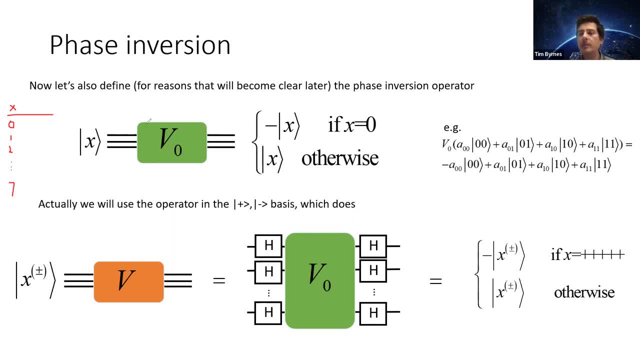 you can have X going from zero to seven because there's three qubits and two to the power of three is eight. If you start at zero, then it goes to seven, okay, And then. so basically, when I say state: 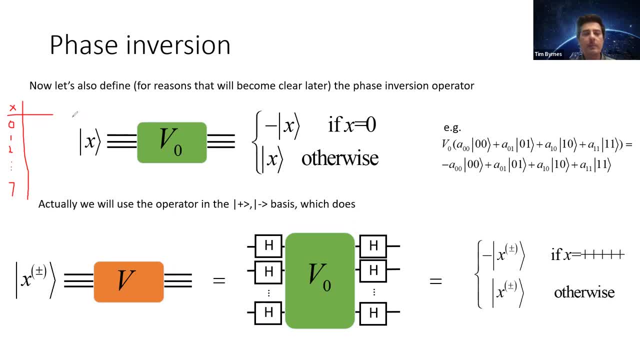 say zero, one, two, three, what that actually means in terms of qubits, basically the qubit decomposition. here is, for example: this would be zero, zero one. sorry, zero, zero, zero. this would be zero, zero one. 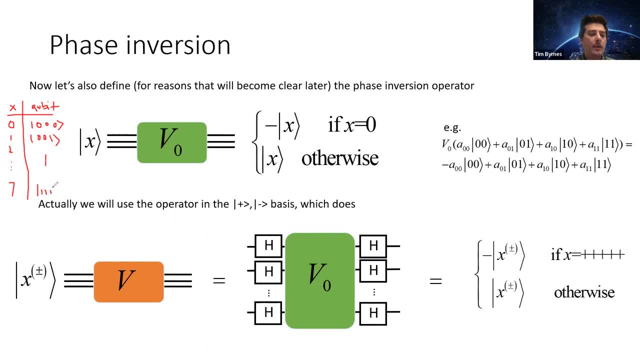 dot, dot, dot, one, one, one, okay. So that's actually what I mean. when I say state X, It's actually like a multiple qubit state, okay. And when I say X equals zero, what I mean by that is that basically. 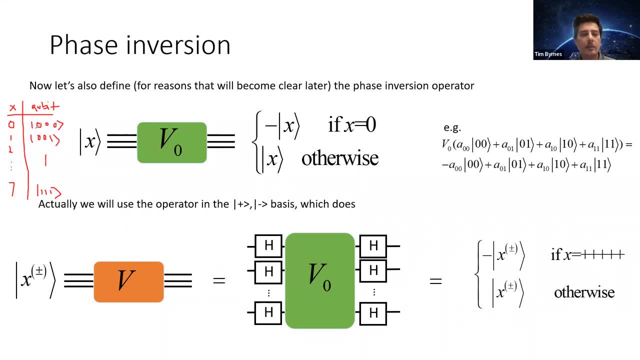 it's the three qubit state, in this case, with all the qubits zero. okay, And basically what this particular operator, V zero- does is to put a minus sign on the state. just the zero, zero, zero state, and then all the other states are left alone. 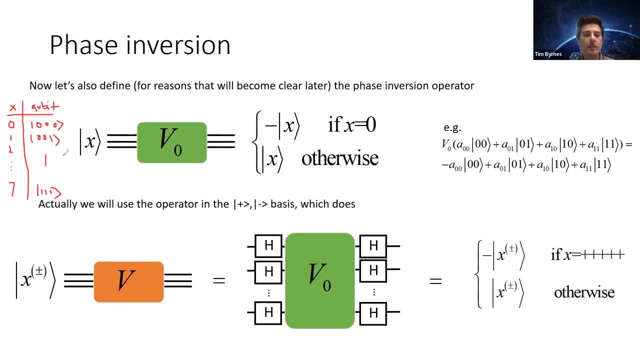 So there's no minus state, minus one phase in front of all the other states here, So this is the only one that gets the minus one. So, for example, okay, here's a two qubit example. So, given an arbitrary superposition state of two qubits. 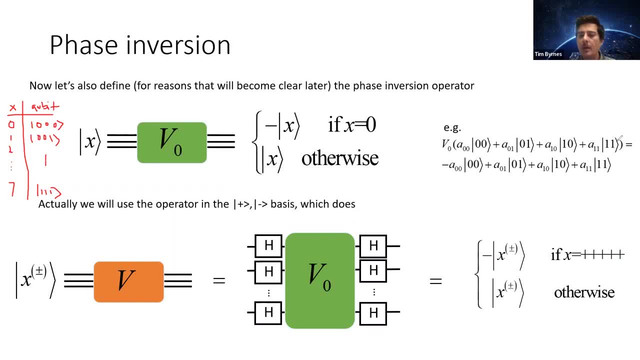 yeah, zero, zero, zero, one, one, zero, one one. basically, what V zero does is just to flip the minus, sorry, flip the sign of the zero, zero state. So there's a minus sign, okay. 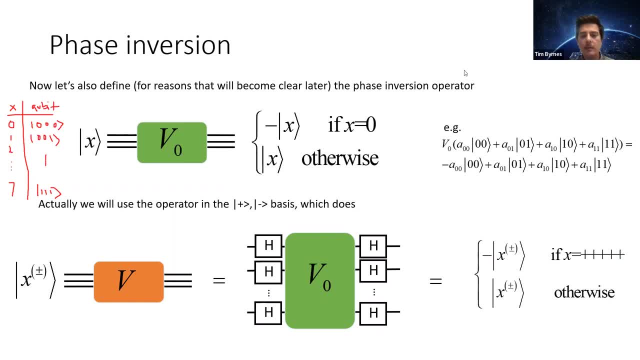 Now. so that's V zero. Now let's do one more extra step on this, and this will be the actual operator that we use Now, if I put Hadamard gates on the start and the end of all these. basically, what this does is to rotate. 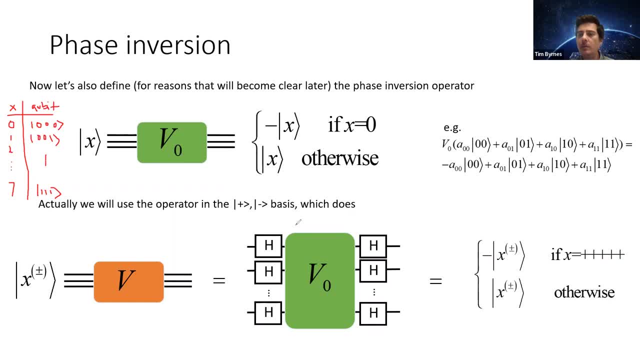 the whole basis, from the zero state to the plus minus base. And so actually, this orange V, this V operator, which I'm gonna define as this thing where I've got these Hadamard gates beginning and ending. Basically, what that does is something very similar to here. 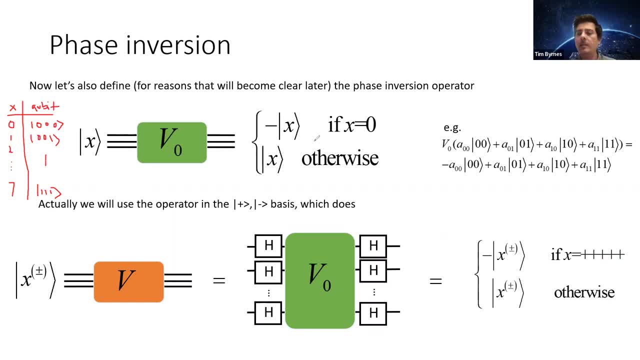 except that I'm working not in the zero one basis but in the plus minus space, And because when you do Hadamard of zero state, you'll get that's equal to plus. So basically, this state here, where you know X equals zero. 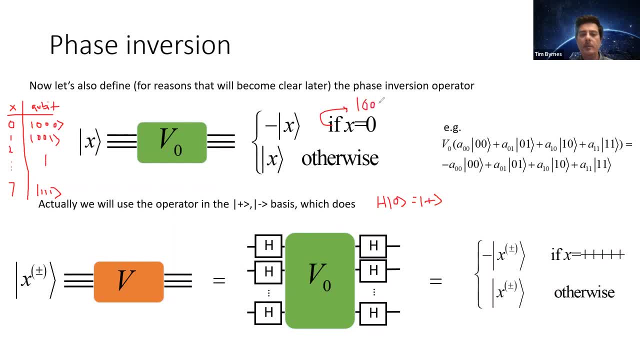 and that basically actually means you know the state which is zero, zero, dot, dot, dot, dot dot zero. basically, instead of the zero state picking up the minus space actually in the state that we'll pick up is the state. 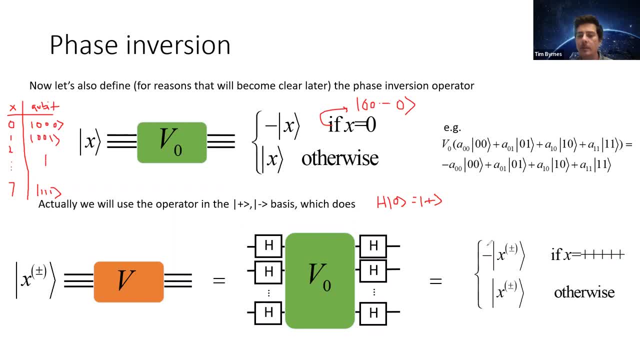 where all these are pluses. So basically, the only state that this will pick, that will pick up a minus state, minus one phase, sorry- is this state where all the states plus. okay, So on every qubit, if every state is plus. 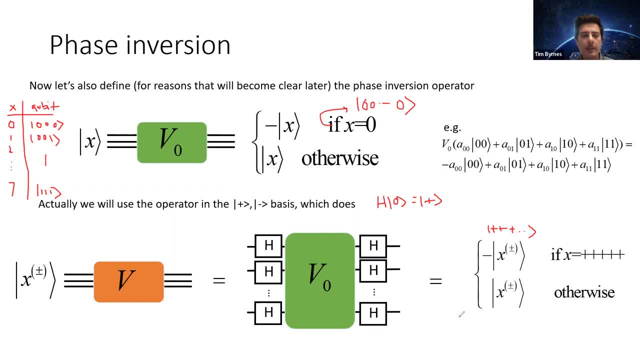 then it will pick up a minus state. Now these other states. what do I mean by the other states? Just like I've had over here? the other states are just all the other combinations. So here's X in the plus minus basis. 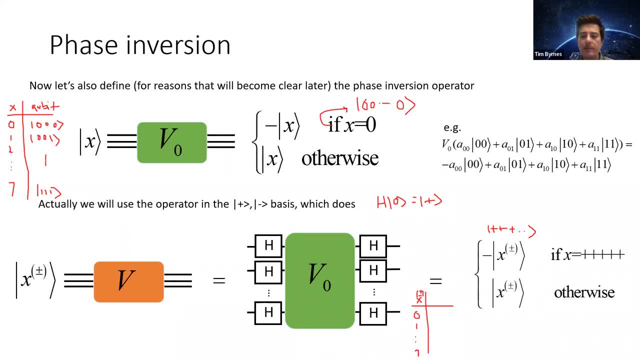 So when I say zero one to seven, what I mean in terms of the states here is that this first one will be the state plus plus plus. Second one will be the state plus plus minus, and then dot dot dot. 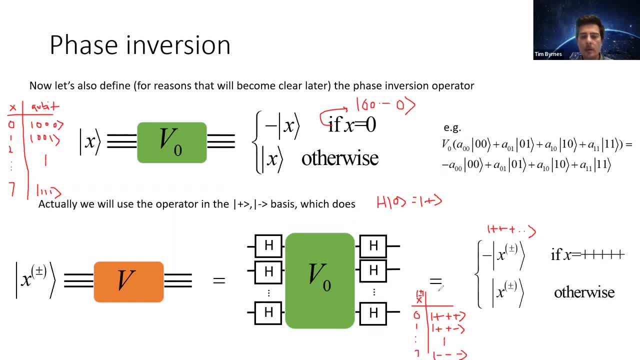 the last state is minus, minus, minus. okay, So in the qubit representation. So basically this state here, state plus plus plus, is the only state that actually picks up a minus sign. Okay, So that's basically what the V operator does. 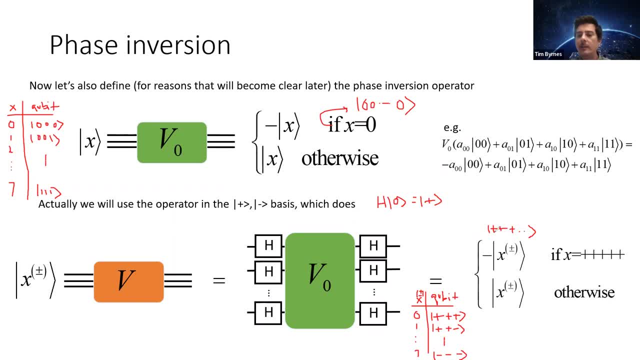 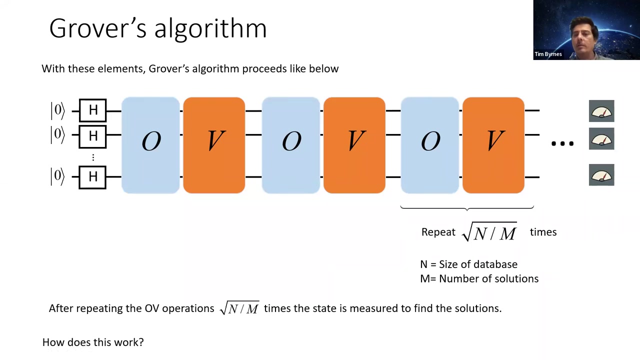 It just applies a minus sign on the state plus, plus, plus. That's fine for everybody. Yes, Okay, great, Okay. So now we can introduce Grover's algorithm. Okay, And so it's actually. it looks pretty simple in terms of the actual algorithm. 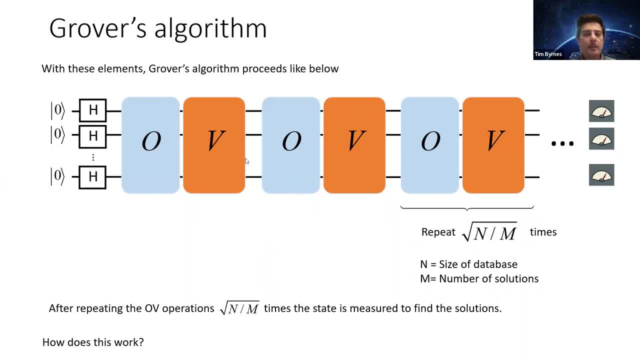 So this is the quantum circuit for it, And what is happening is that? okay, so the initial state is just a zero state, Okay. And then you initially apply some Hadamard's. Okay, So at this point here the state will actually be the state just plus, plus, plus. 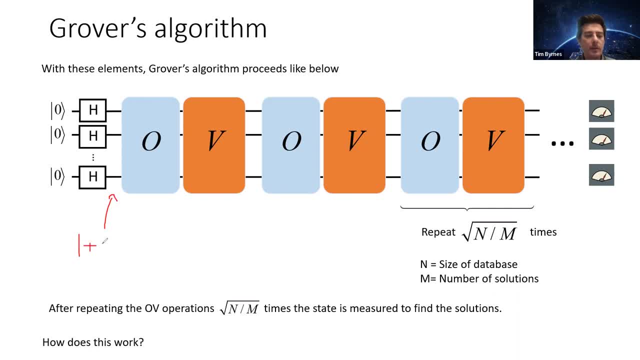 So over here we're going to go through this, I think. so over here we're going to go through this, I think, in detail, But over here it's plus, plus, plus, And then after that we just apply the O and the V operators. 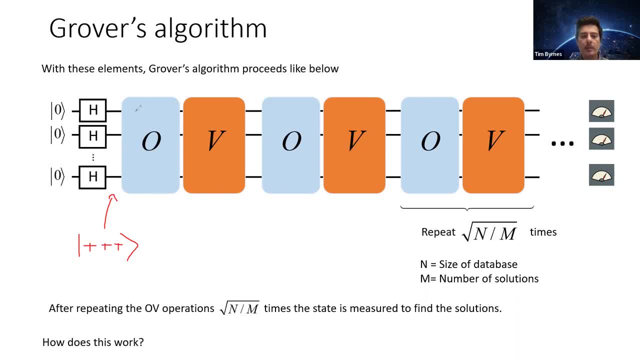 Remember this: O is the oracle, So that's the thing that applies the minus signs to the solution states. Then V is just the operator that applies the minus sign just to the plus state. Okay, So actually this state here, And then you just repeat this. 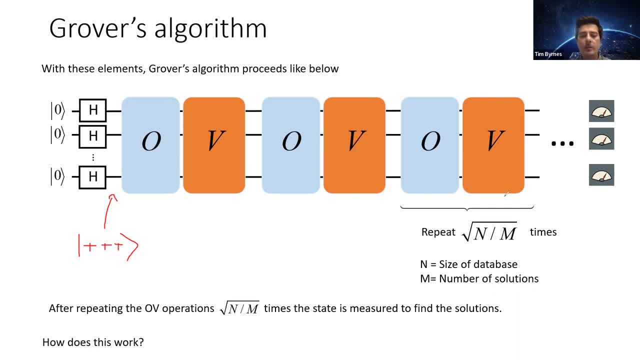 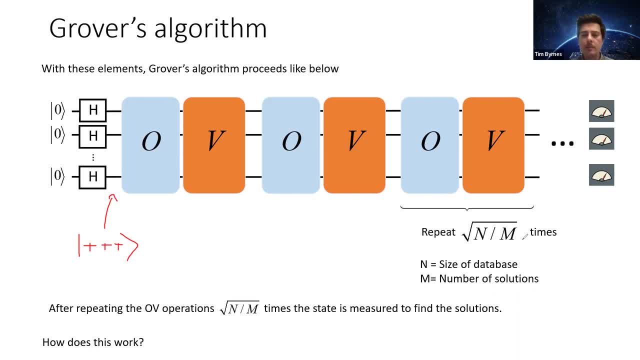 And also depends upon how many solutions there are. So, for example, in the example that I had before: okay, how do I go back? I'll go back. Oh, here we go. Okay, yeah, In the case that I had before this M. in this case, 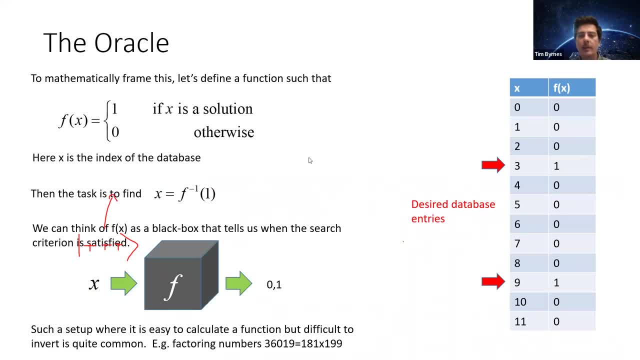 but, for example, just to tell you what the N and the M is, here is the N in this case would be, for example, 12. That's the number of database elements, And then M would be the number of solutions, And that would be two. 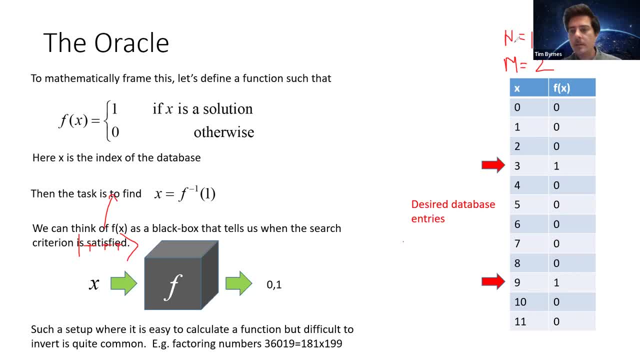 And the M is just two, And so, for this particular case, this M is just one value, and I'm mixing them up. So here we go again. we're going to do this type of thing. It's going to be V M. 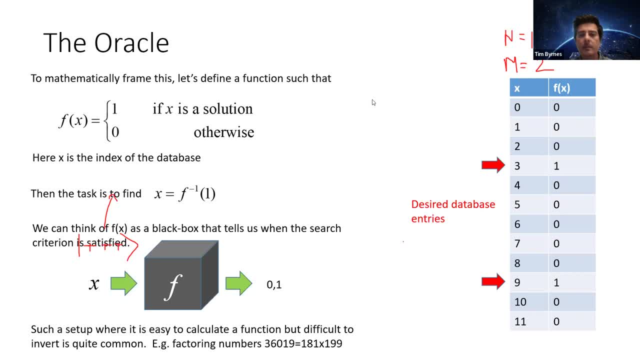 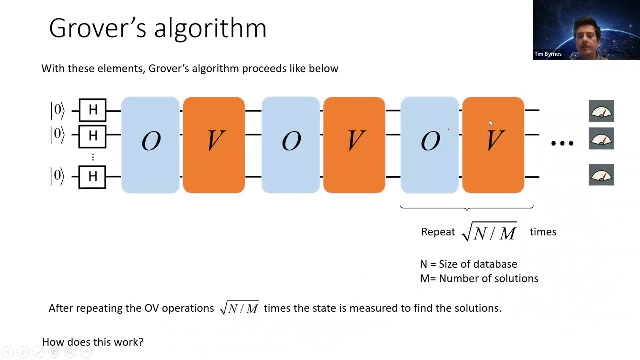 and then just this M, and then the X and Z- they're going to be the same values- And then this one will be this M, and then this M, and this one will be Y M, And this one will be this and this Y M. 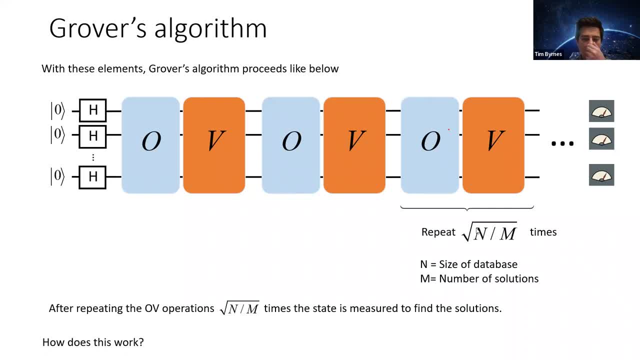 So that basically specifies the. these are kind of two parameters that you have. And well, just delete that number of times which is n over m square root, okay, and once you've done that, you measure, you measure the qubits and if you do that, when you measure it, basically the output of the circuit. 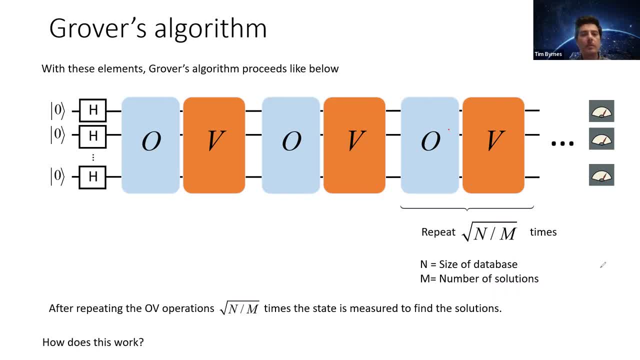 should be one of the solution states. okay, so you just read off the solution state. so, uh, you know, perhaps the solution state is, you know, like you know, say, say it's that state, so you know, whatever. you know, whatever that is in binary um, you just read off the values. 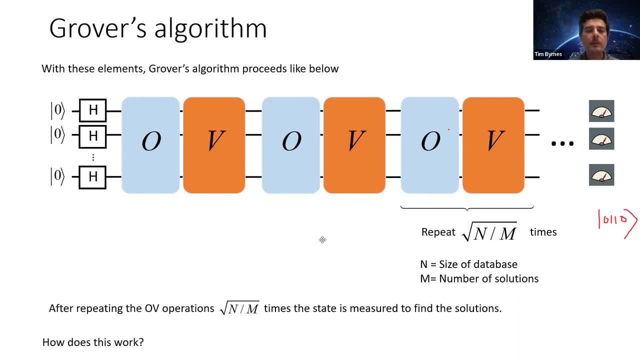 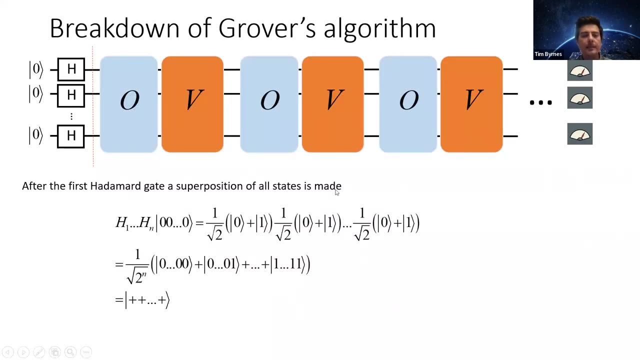 okay, so that's how it works. now, um, you know, i'm sure this doesn't this looks kind of mysterious. um, you know what? why does this work? so let's, let's dive into that. so, um, so, let's go through it step by step. so, as i just said, um, after the hadamard gates, basically. 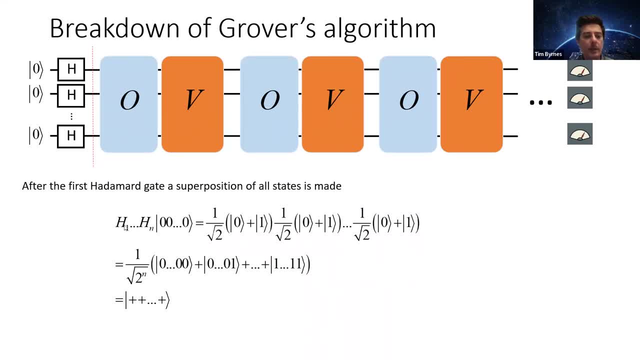 what you'll have is this state where you've got hadamard applied on these zero states and that produces the plus state. okay, and so here's a plus state, here's a plus state, here's plus state. now, if you expand all this, so you know, you can write. 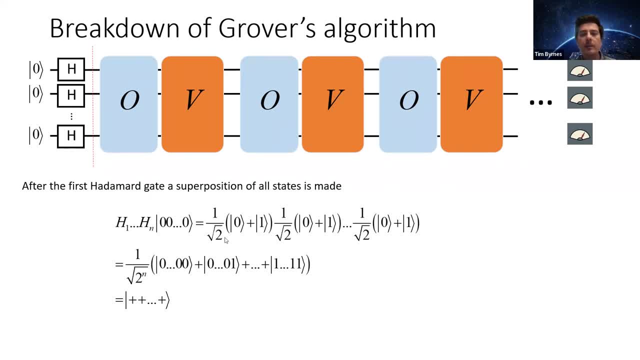 it like that, that's perfectly fine, but another way to think of it actually is: if you expand all these brackets here, then what you're going to find is that, well, you'll have actually every single possible combination of states. okay, so, uh, you know, you'll have every state here, going from zero, zero. 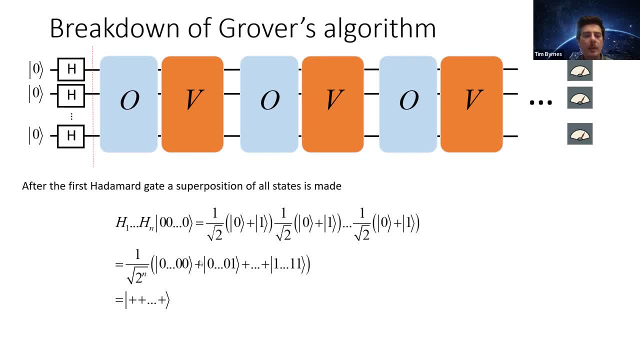 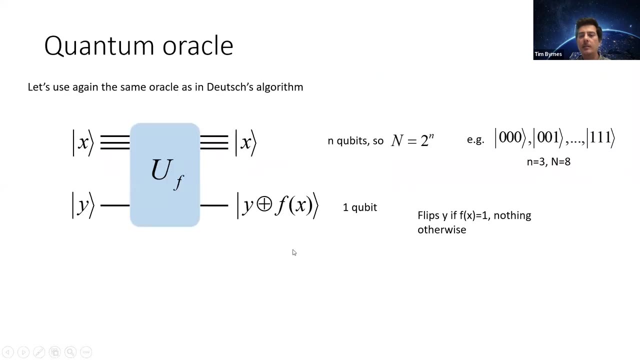 zero, zero, zero, zero all the way up to one, one, one one. so actually this state plus, plus, plus uh- is actually an equal superposition state of all the potential different database entries. so basically it's like you know, in this table here you're starting off with a superposition of every. 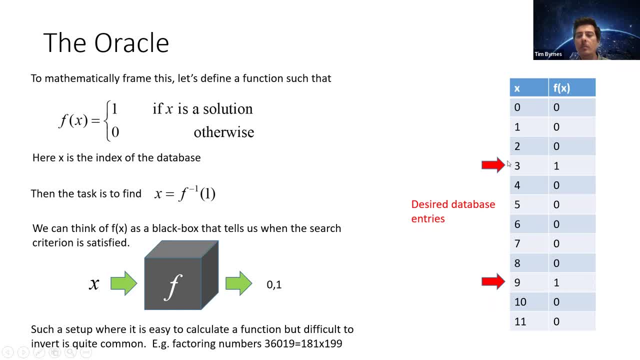 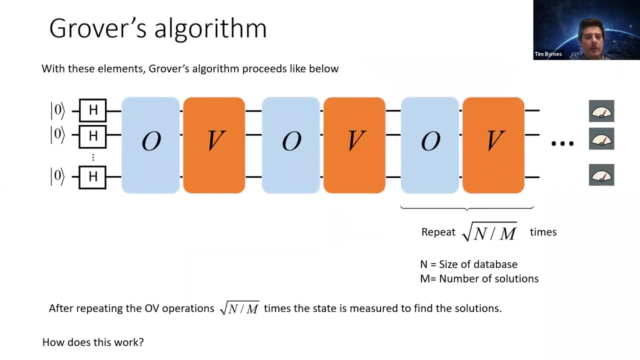 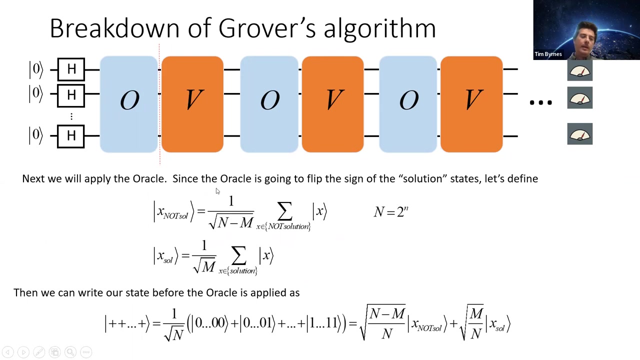 possible entry, okay, and we, we don't know which ones are the solutions yet. so in this case it's like three and nine, but the starting state is just a superposition state of all of them. okay, so that's the first step, okay, now, uh, let's look at what happens when you. 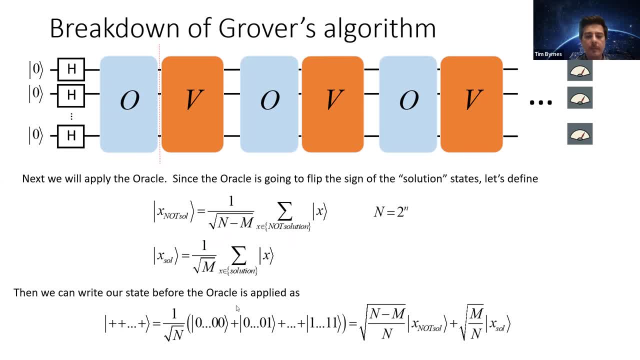 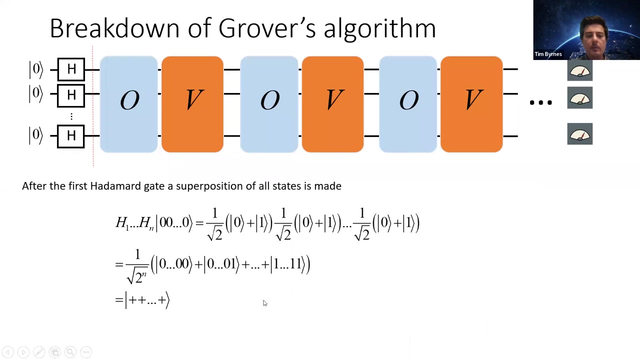 apply this oracle state once. okay, so remember, what the oracle does is to just apply a minus sign on the uh solution states. okay, so, uh, you know, um, well, uh, so, for example here: uh, you know we're starting with all the possible potential solutions, yeah, and basically, uh, what it does is it's going to flip after this first. 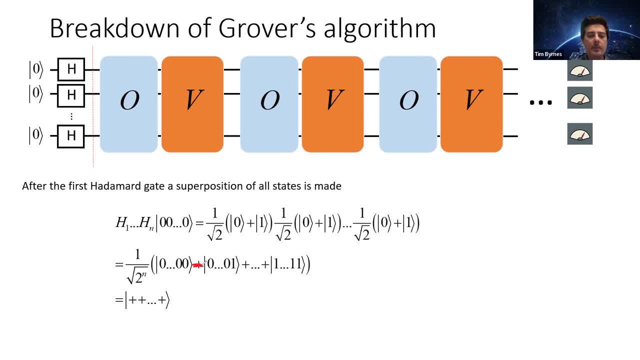 oracle, here you flip the sign of one of these. so imagine if, like this guy, zero, zero, zero, zero, zero- one is say this one of the solutions, it's gonna, it's gonna flip that sign to a minus and it's gonna be a minus sign. and if there's only one solution to the whole, to the whole database, then that's. 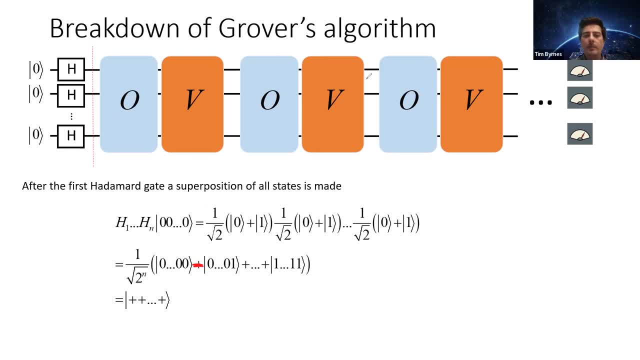 the only term that gets flipped, but if there's more than one solution, then there will be uh, multiple, uh spin flips. so maybe, like this, last one is also a solution, in that case that will also have a minus sign. all the other ones that are not solutions will uh remain the same in the phase. 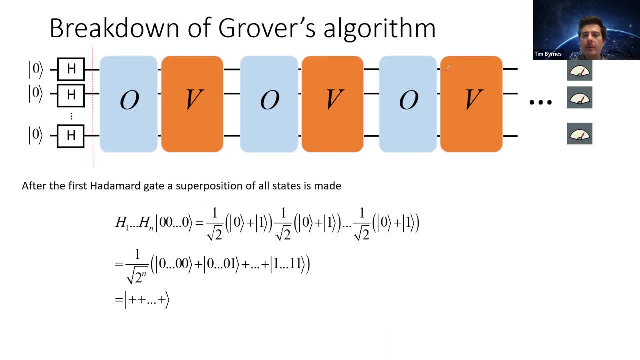 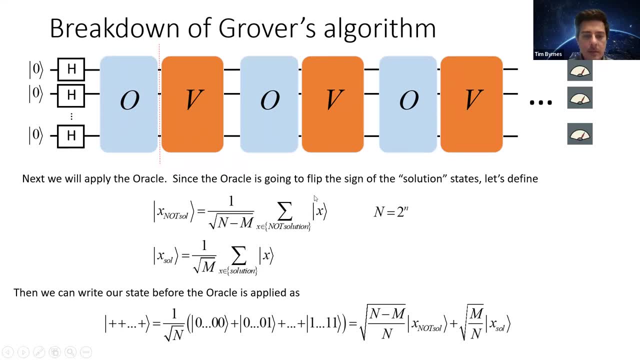 okay, just have a plus plus phase. so the way to write this, uh, more generally, is like this: so, uh, suppose we have um here the set of all the states that are like not the solution, right? so, um, you know, all the cases that do not satisfy fx equals to one. this is, uh, it's basically this part of it. 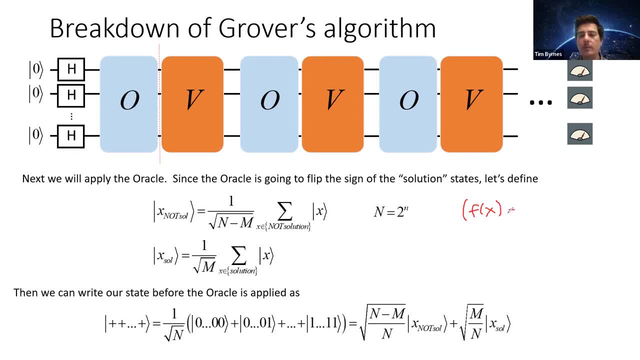 fx is uh not equal to one, or of course it's zero. so these are all the x cases that satisfy that, and here are all the cases that uh do satisfy that. so this is: fx is equal to one, okay, okay, and so long so that we actually can norm, normalize the state. uh, here's the normalization. 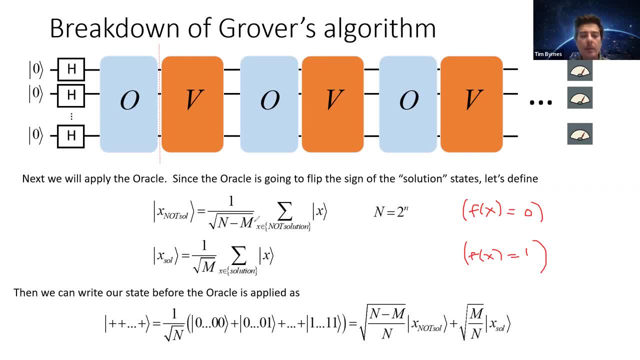 factor: well, the number of cases that uh have that are not in the solution. well, n is the total uh database size and m is the number of solutions. so obviously the number of not solutions uh is like n minus m. okay, so this is why the normalization factors like this: over here, the number of solutions is just m. that's how we. 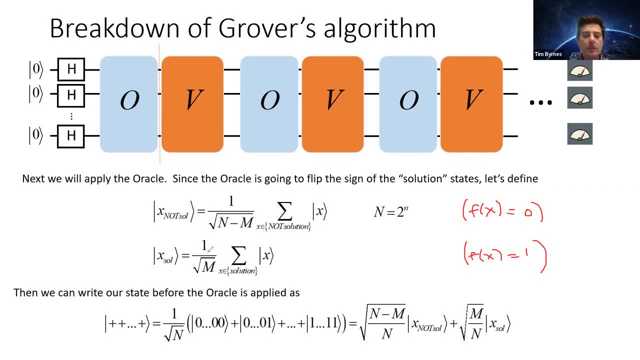 defined m, so the normalization factor is one over square root of m. so that's the number of solutions and uh, so it's actually uh, what we're going to find? is that actually, uh, writing it in terms of this state, which is like the sum of all the states that are not a solution, or some of the states which 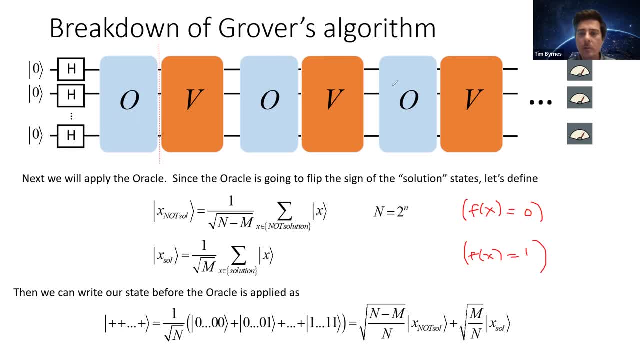 are a solution. this is actually, uh, quite a good way to write it, so what we're going to do is: let's just go back to this point in the circuit, okay, so let's write this initial state, which is this, which is the state which is a superposition of all the possible states. let's write it in terms of uh. 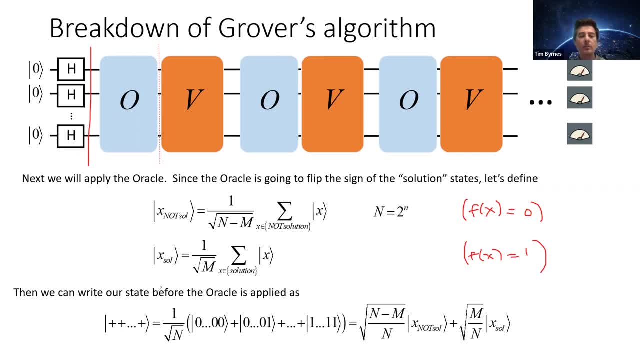 these two vectors here. so the x not solution and the x solution now um. just with a little bit of rearranging, uh. you know, if we multiply this uh by square root of n plus n minus m, then we're going to get um. you know well, the sum sum over x. so x in um not. 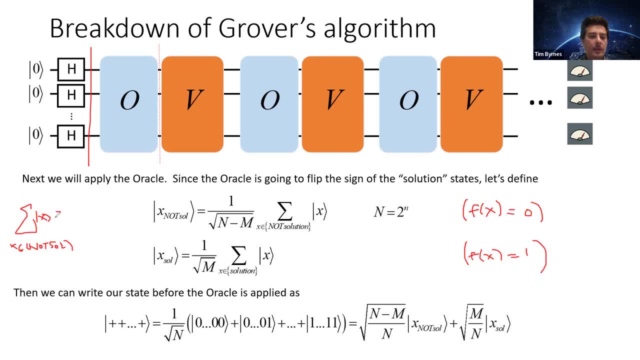 not solution um. so this will be equal to square root of n minus m. i've just rearranged the this equation, uh, where it's uh, x, uh, not. okay, i'm just going to call it x, not, and then, over here, this is this: uh sum of states that. 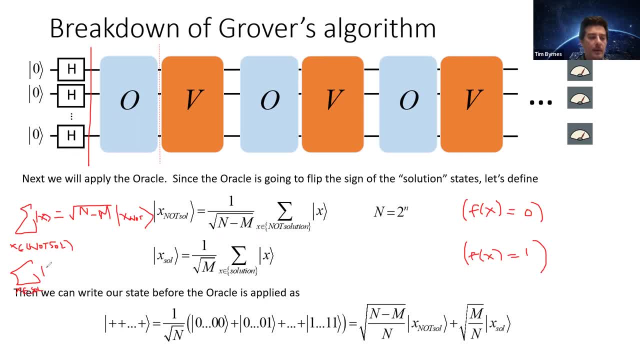 are in the solution. so this one, uh, what we can do is we can. uh, this one is going to be called multiplied by square root of m. let's just put this on the other side. so these are the solution states, okay. and then, um, if we wait a minute, uh, oh, yeah, so that's right, okay, and then, because this state here actually, 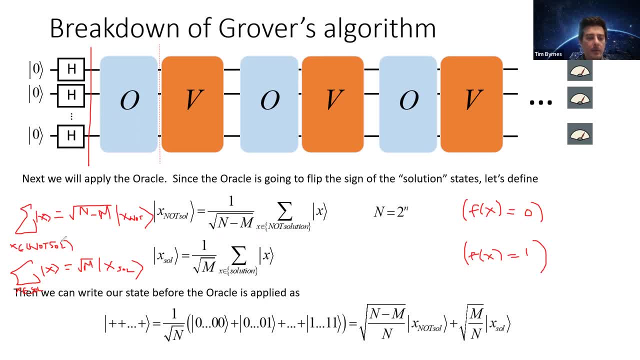 has this normalization of one over square root of n. so what we can do is that this stuff here is actually equal to, uh, basically the sum of these two guys here. so if we add basically these two, two states here, that's the inside of the brackets, and then we, if we, 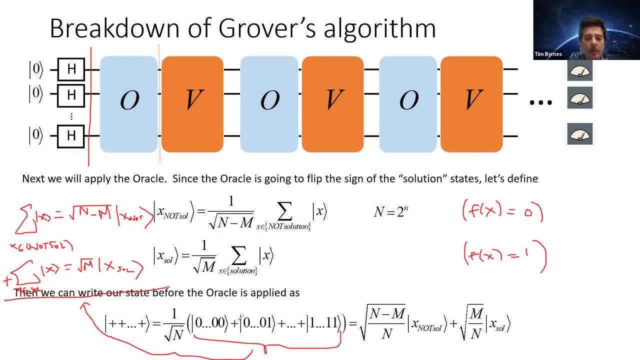 just substitute this guy, uh, into here, and then this guy into here, then we're going to get, basically, this is the equivalent way to write this state, which is, uh, some sorry, the the initial plus state. so remember, this is the state just before the oracle. okay, and if we write it like: 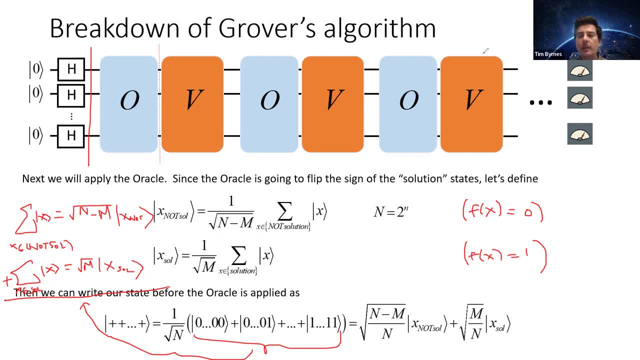 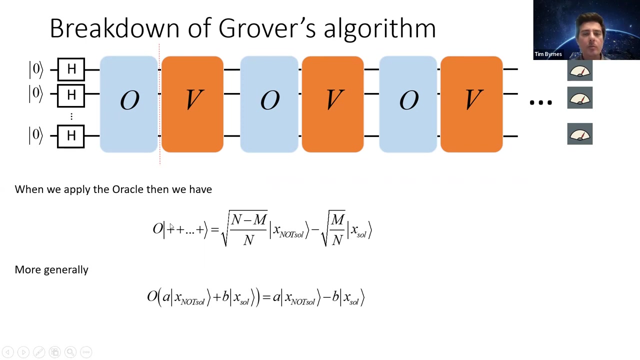 in this form: um, makes our calculations quite easy because, uh, so everybody, fine, i'm going to erase this now- is that fine? yep, okay, all right. so if we write it in this form, and it's easy to see what the oracle does, because when we apply oracle to this initial plus state, then remember what the 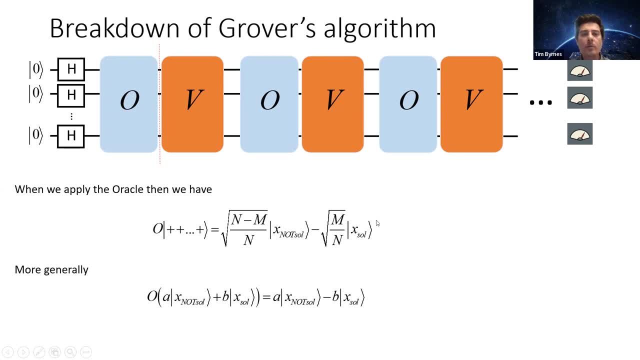 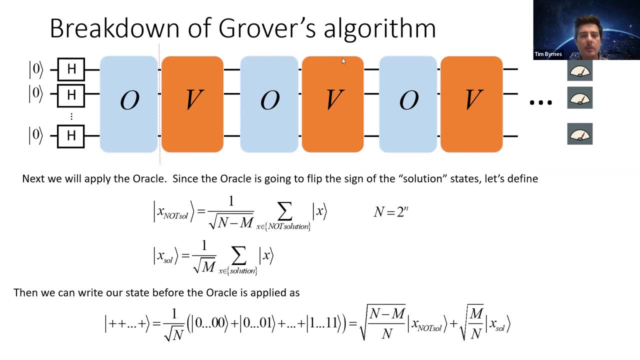 oracle does is to add a minus sign to all the solution states. okay, so it's just going to flip this sign. so just to emphasize what, what, what has changed here, here's a plus sign over here. That's the state before the oracle and state after the oracle has a minus sign. 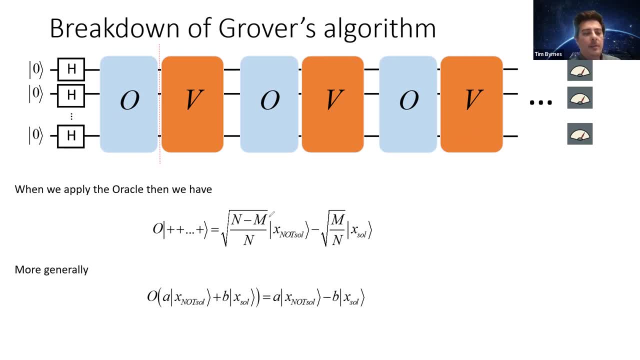 So that's what happens after the first step, And well, in general, basically that's what the oracle always does: Just flip the sign of this term here. Okay, then let's keep going. And then now, oh, I see, yes, sorry, 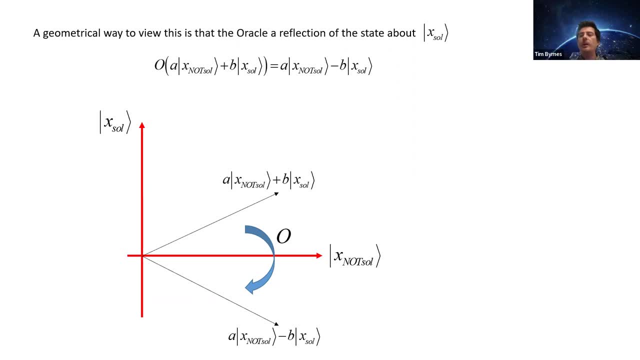 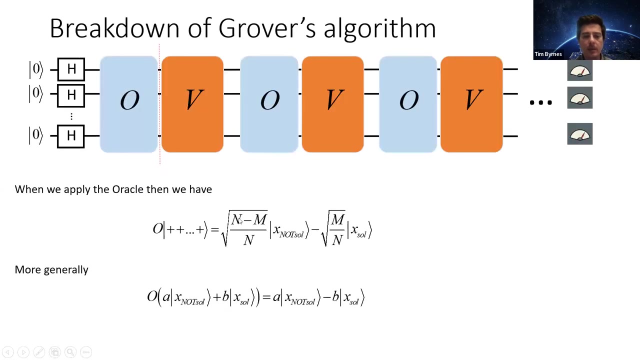 There's a really nice way to actually visualize what's happening here And let's plot this state, this general state, here. So actually in the first step, we've got particular coefficients of N minus M over N root, M over N root. 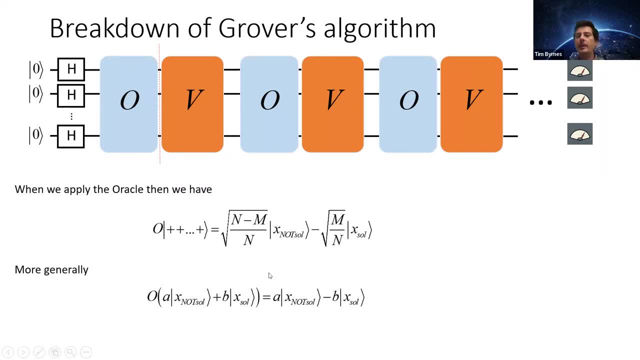 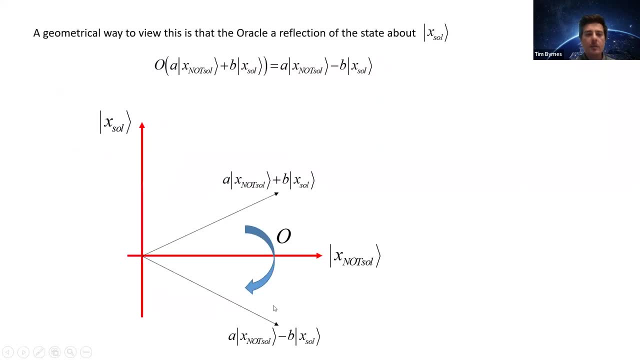 But let's just look at this more general case first and just try and get a sense of understanding of what this oracle is actually doing. So what it's actually doing is, of course, so it's flipping the sign of this B, but we can visualize this geometrically. 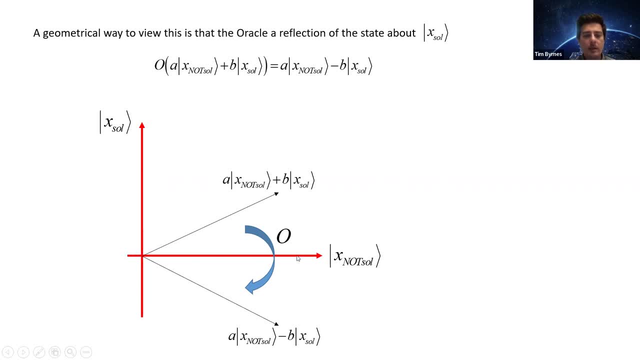 And the reason why it's doing this. it's because so this original state here, which is A and B, so some arbitrary coefficients And the axis here. let's consider these. here's the X- not-solve state And here's the X-solve state okay. 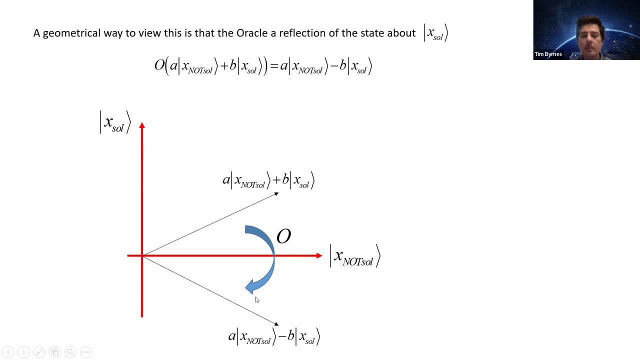 So what O basically does is to reflect around this X not-solve axis. okay, So because O is not a prime, right? because after you apply this oracle, this has a minus sign. So whatever it was up here, it will be reflected around this axis. 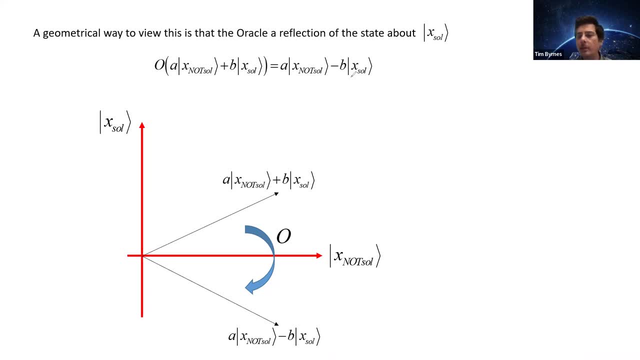 And so I'm kind of thinking like A and B are real numbers here, And in fact what we're gonna see is that actually, throughout this whole thing, the coefficients of A and B are just always real numbers, So we don't really have to think about. 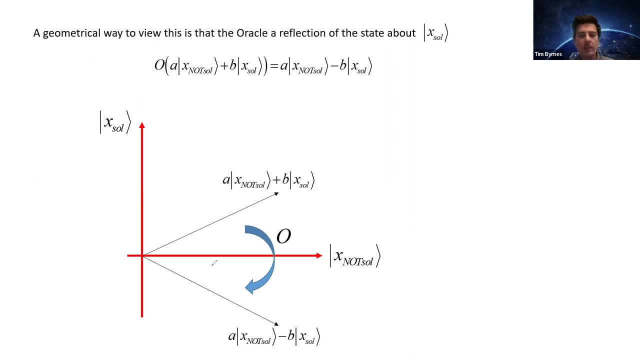 the measuring components of A and B, So it makes our life a bit easier. So we know it's definitely a reflection because basically the coordinate here is A and coordinate here is B, And of course the coordinate here is minus B, Coordinate here is still A, of course. 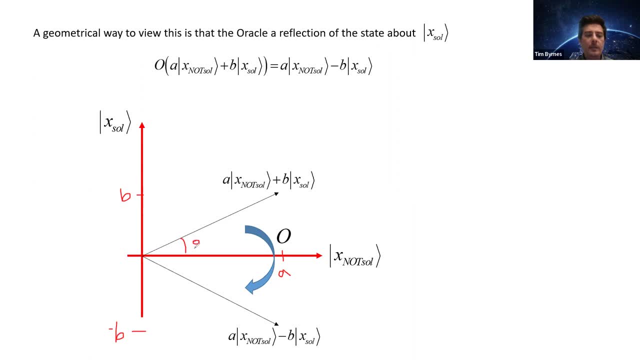 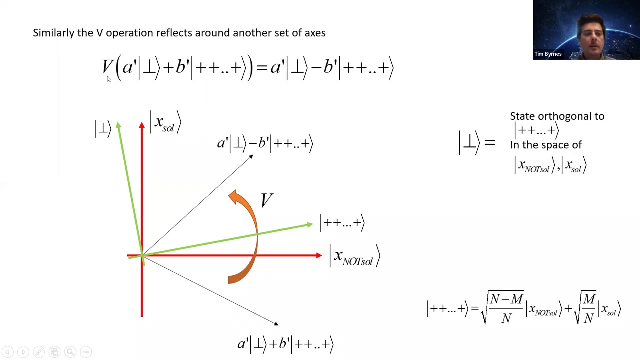 And so obviously it's a reflection. So this angle here is the same angle. So this is a really neat way of visualizing and we're gonna make use of this because we can actually use the same trick to understand basically what the other operator here B, actually does. 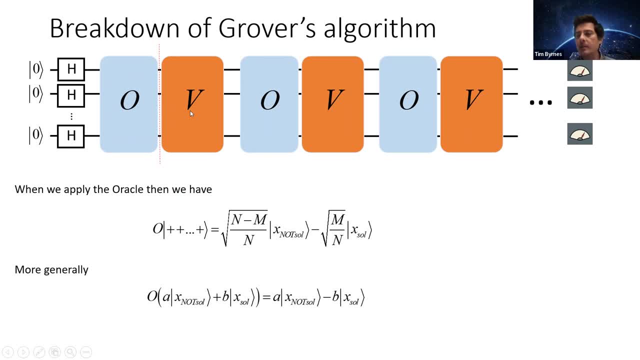 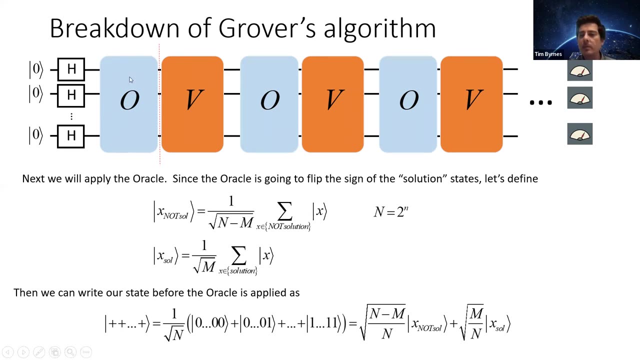 So remember, O and B are just about the same thing. I mean sorry they're not the same thing, but uh, they're very similar operators in the sense that o is something that adds a minus sign to the solution states, and then b is the operator that adds a. 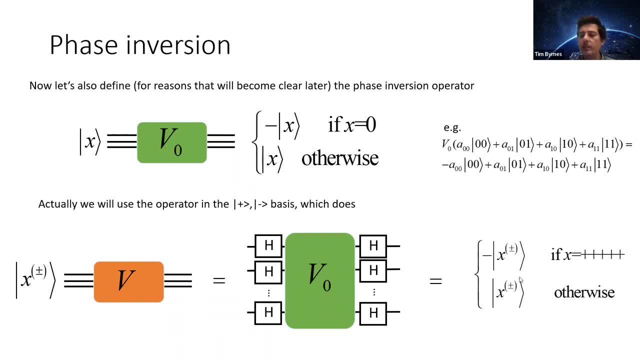 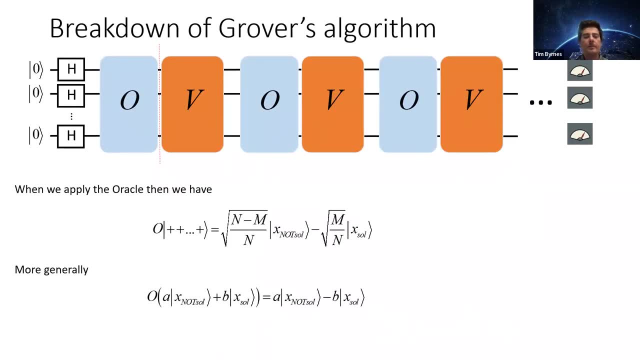 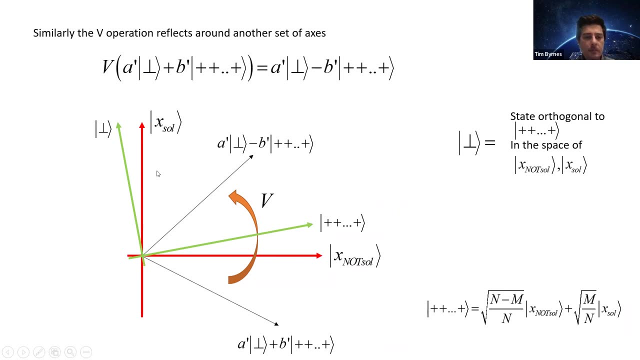 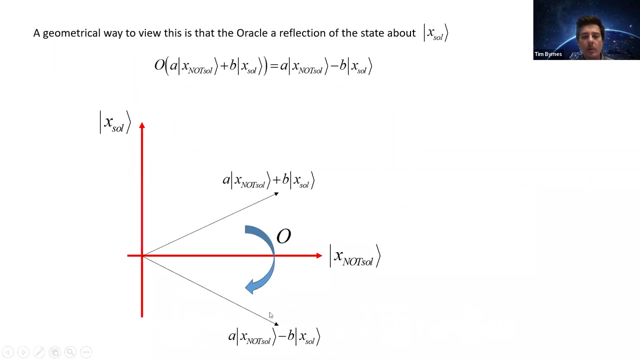 minus sign to the plus state, okay, so all these states plus. so you know, kind of they're just, you know sort of similar kind of things. so we can actually understand what the v operator does because um, uh, basically, uh, if you think about o as um, applying, basically performing a reflection. 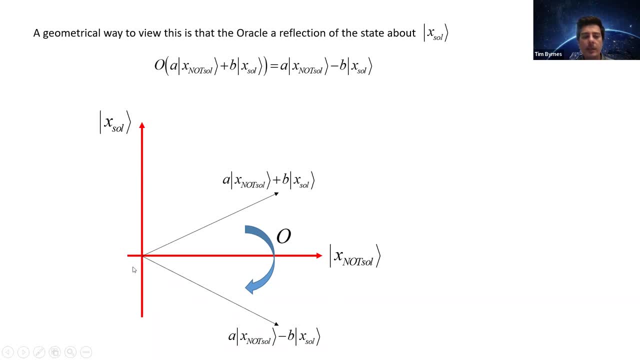 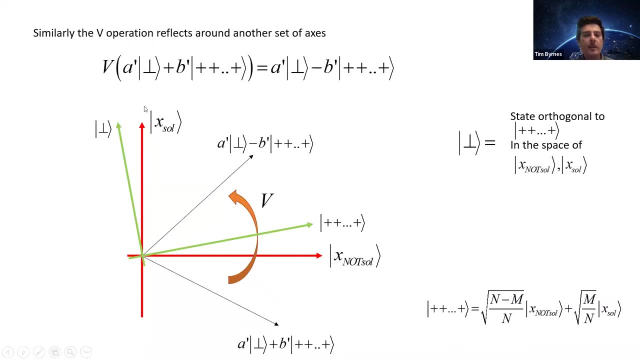 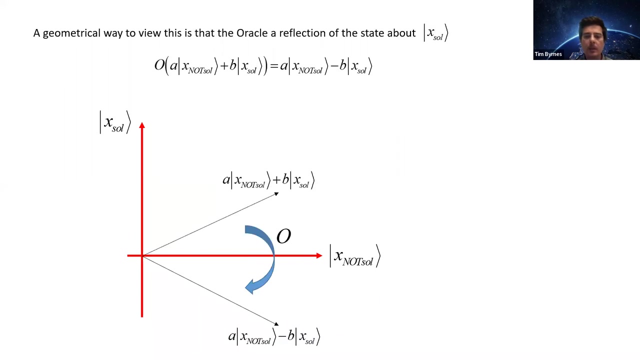 around about the uh, this state that does not have the solution. okay, so because v is something that actually um, okay, maybe it would have been clearer if i actually put the minus sign. so over here, the yeah, okay, it might have been a bit clearer. it's actually the same thing, but. 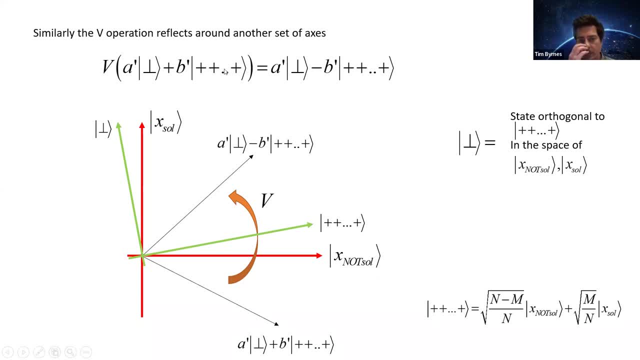 uh, it might have been a little bit clearer if i define this in the opposite way in hindsight, but uh, so because b is the operator that uh applies a minus sign to the plus state. um, we can also visualize v as being a reflection uh around the the plus state. actually, okay, so basically the role of the. 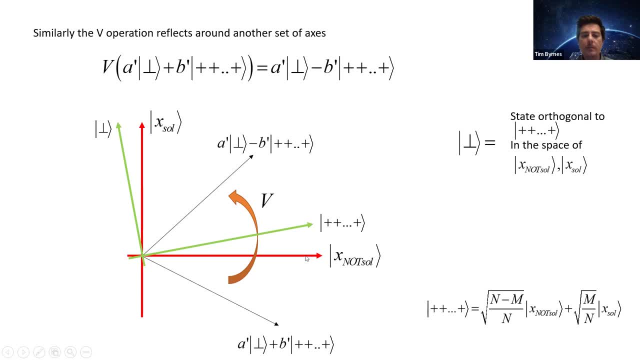 bus state is playing the role of the uh not solution state that we had for the for the oracle. okay, so the in the in the case of the oracle, uh, we were, we were doing a reflection around not's fault. and for v, we're performing a reflection around the um, the plus state. 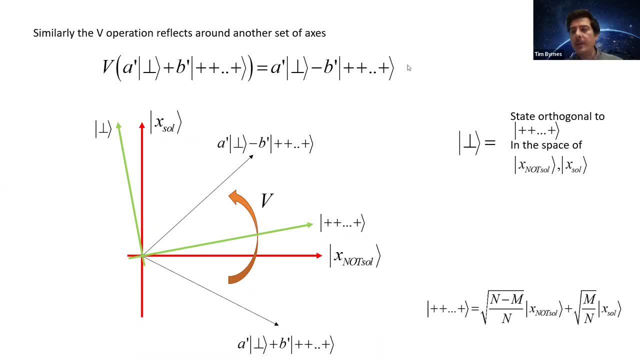 um, and i mean, you can show this mathematically, but it's a little bit tedious because it's actually, uh, you know, at around these green axes and the green axes are not, you know, it's not not the same angle as the, as the, as the red axis. okay, so i remember trying to. 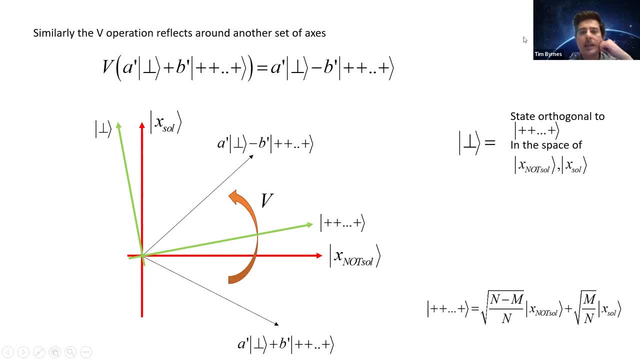 when i was trying to, you know, write these slides, um, i tried to also do it mathematically and then i it just looked very confusing and, um, i think this is actually a much clearer way to explain it. that is, the action of the v operator is just to reflect around this. um plus plus state okay. 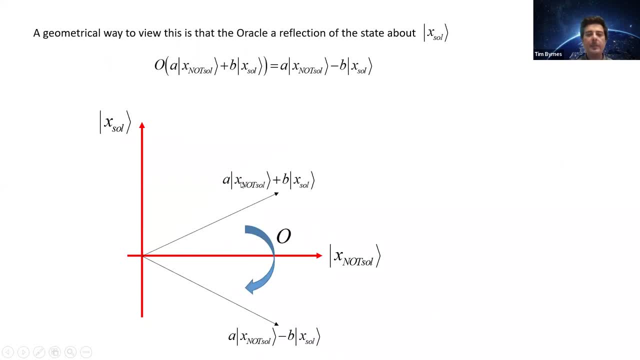 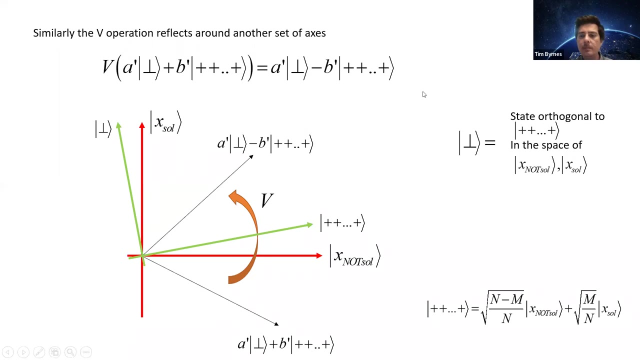 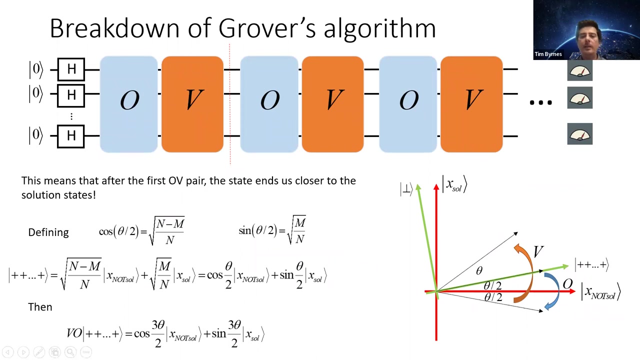 so, uh, i hope you can just sort of see that, because basically the v operator and the o operator are, you know, very, very kind of similar types of things. okay now, um, actually, just with the knowledge of these two things, we can actually already uh deduce basically what's going to happen in this whole circuit, so we don't have to really continue. 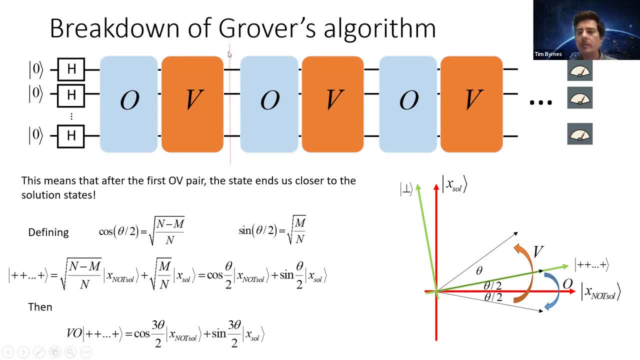 further in this whole sequence. um, of course you know, if you try to do this algebraic maybe you'll start to get kind of messy, so, uh, so let's look at basically what happens after applying. firstly, just you know a single pair of this o and the b. okay, 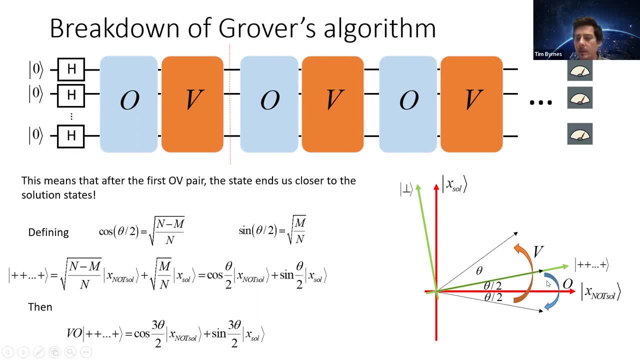 so, uh, let's first look at this picture, because it's probably the easiest thing. so, uh, basically, we've got kind of like these two uh pairs of axes where, uh, you know, the red one ones is the solution and not solution, and then the green one is this plus state and then the state. 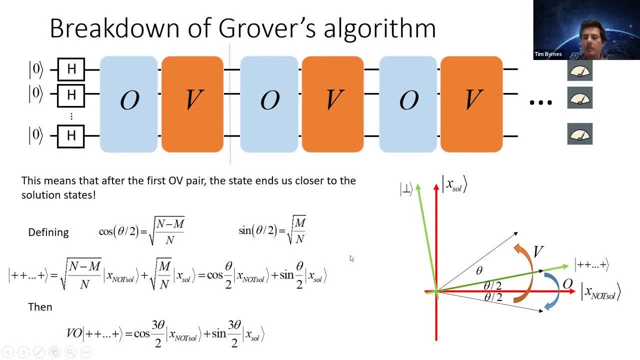 which is, uh, orthogonal to this, plus state um, but in this two-dimensional space. okay, so, uh, so those, those, uh, those vectors are fixed. so think of them as, just like the, you know, two sort of coordinate systems. okay, so there's the red coordinate system and then the green one. okay, 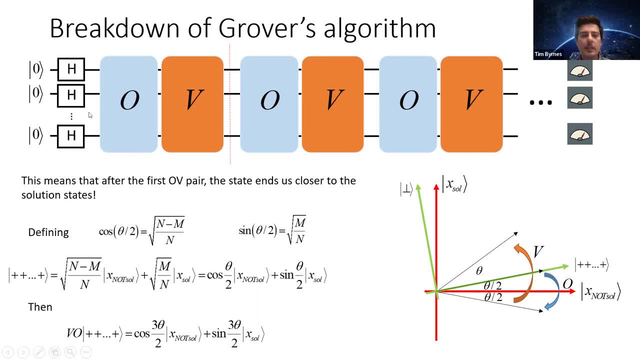 uh, these black vectors are going to be like the state that evolves, uh, during. you know the sequence of this algorithm. okay, so the initial state is going to be along this diagonal green vector because, as i said here, the state here is the state. that's all plus okay. 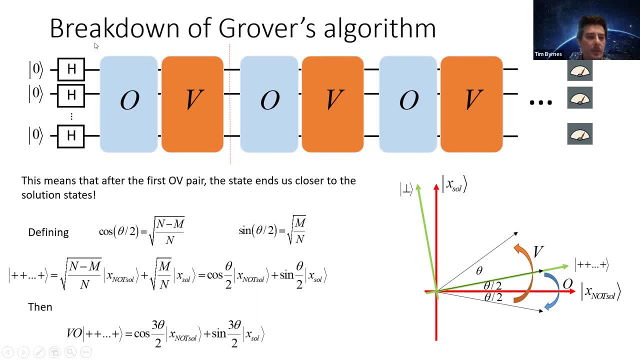 so here's the initial state: uh, at this, this position. okay. now, after the first o, what's going to happen is that it's going to end up down here, okay, it's going to end up, uh, beneath the- uh- red axis, and remember the whole, the whole thing that we're trying to do here. 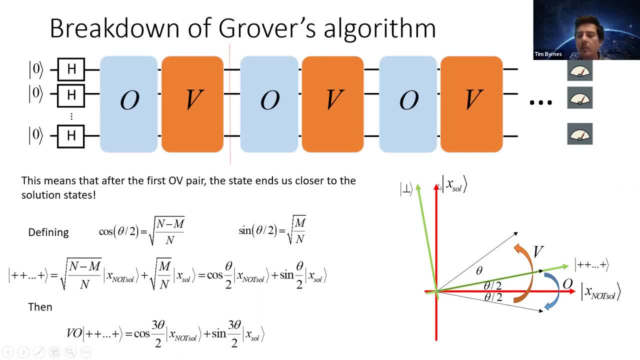 is actually to swing this vector actually towards this, this state here, x, sol, because once we've got found this xol, that's basically what we're trying to do in this whole algorithm. we're trying to get the state in this quantum computer to swing towards this uh, state xol. okay. 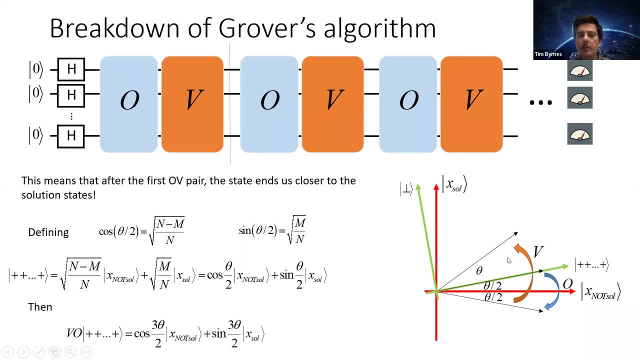 so actually, in the first step, it actually goes the wrong way. okay. so after doing o, it's actually going the wrong way. uh, it's actually further from xol than than it was. uh, initially. okay, uh, but when you apply the v and remember, what this does is to then perform a reflection not around the red. 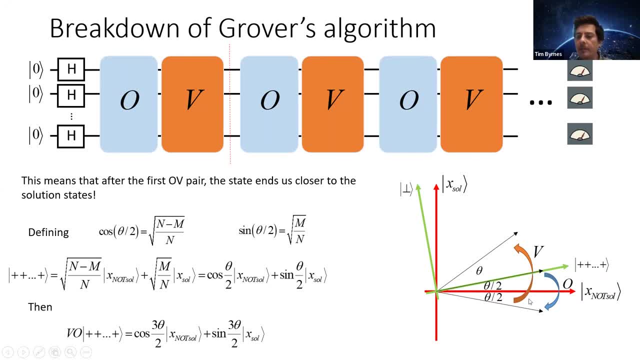 axis here, but around this green axis here. okay, so after the first o it's down here, but after the first v it actually gets reflected this way and this time, actually, it ends up like this: so it's going to end up being closer to the xol than it started with, okay, so basically this pair: 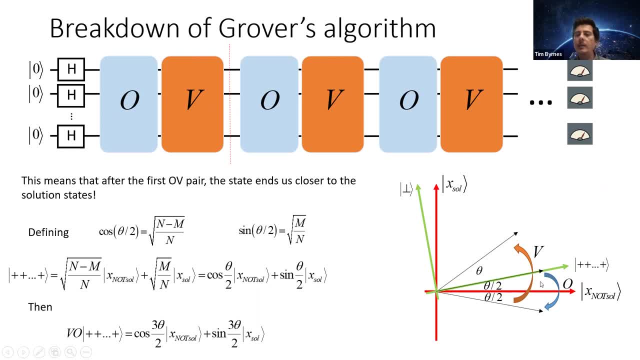 of operations: o and then b, uh will actually uh, swing this vector closer to this xol vector than it was initially. um, now, if you repeat this, you can actually figure out what's what's going to happen. okay, because maybe a different color here. so so now the vector's here, right, okay, and then so we're. 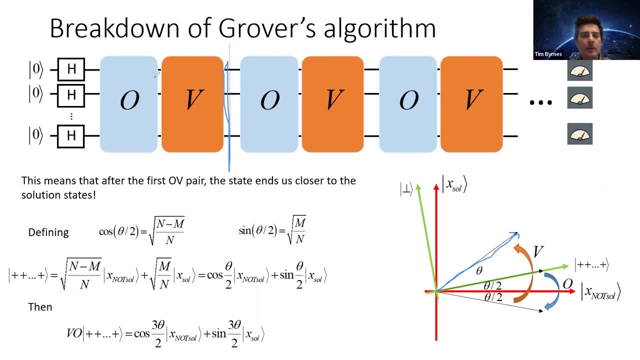 we're at this point in the circle, okay, so after one iteration of ov, the, the vector is here. uh, the next o is going to reflect this blue vector here around the red axis, okay, and so this angle here is going to be three, three theta over two, so actually it's going. 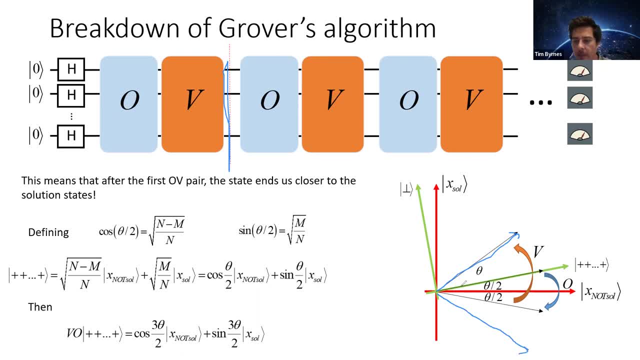 to end up over here, and this angle here is going to be three theta over two, okay, and then, uh, this v here is going to reflect, uh, the, this blue vector around now, this time, this axis, and if you look at the, uh, did i do this right? no, i didn't roll, sorry, let me. 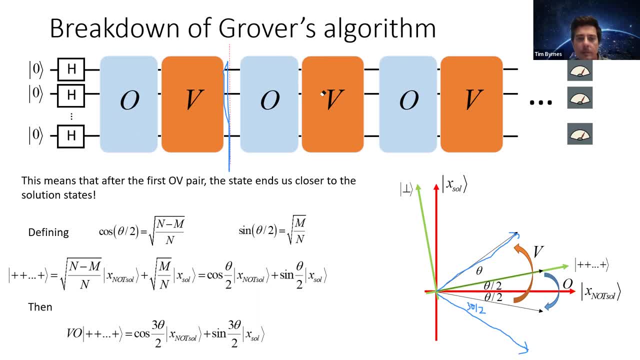 try and fix it up. uh, so okay, so sorry, start. this is where we start at this point. and then the angle from here to here is three theta over two that. so, actually the angle from here to here is three, three theta over two. okay, then now we're gonna. uh, the second v here is going to reflect this blue vector around this time. 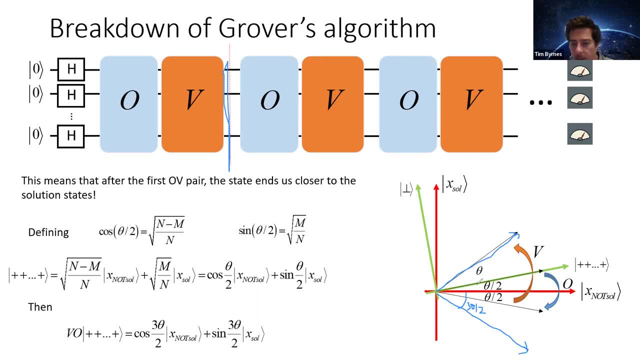 this green axis here, and then the angle from here to here is actually two theta. now okay, because it's three theta over two between the blue vector and the in this red axis, and then this angle here is theta over two, so that's two theta. so actually, where this will end up after the second v is actually going to be. 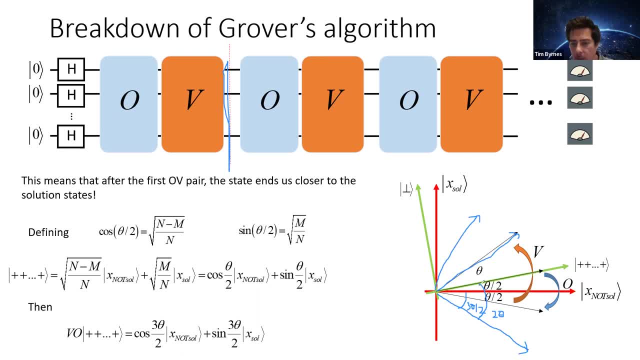 uh, over here and from here to here, it's two theta, and then from here to here, it's going to be also two theta. okay, so if we track what's happening to this vector, so in the first- uh, you know, let's let's look at the angles. so in, in the initial state, the angle was theta over two. 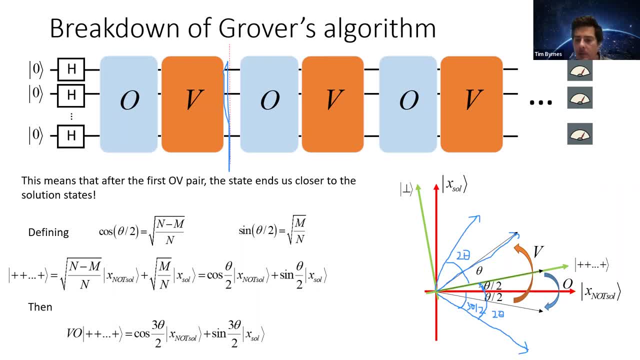 and then over here the angle was um three theta over two, and then over here angle is five theta over two. okay, So basically, each time you apply this OV it gets closer and closer to this X sol. Actually, if you keep on doing this, it can overshoot okay. 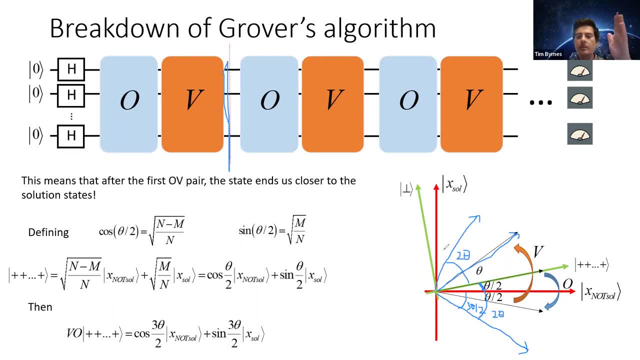 So it'll. if you're wondering, you know what happens when it's finally actually gets there and then you keep on applying OV. actually, it'll just keep on going. Actually, it'll just keep on revolving. So this is why you need to actually stop. 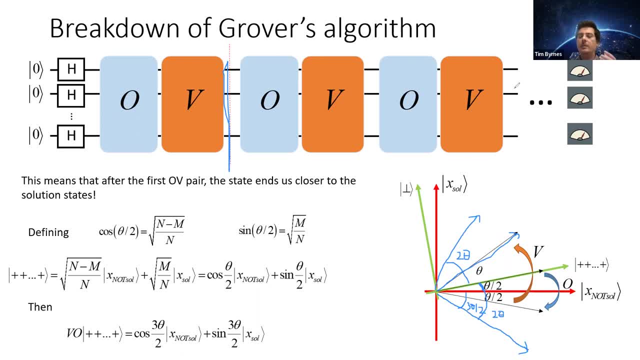 and then measure when you actually applied it enough times. Okay, so I'm gonna explain the maths now, but basically that's really what's happened. Any questions you guys have? Okay, well, stop me if anything's confusing. So mathematically, this is how we kind of derive it. 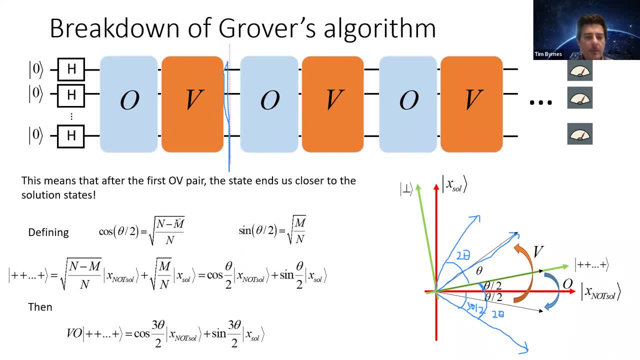 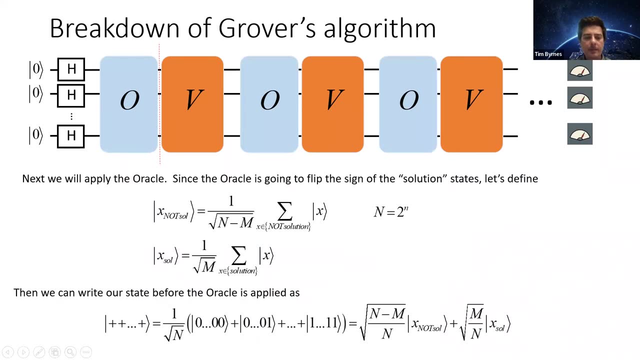 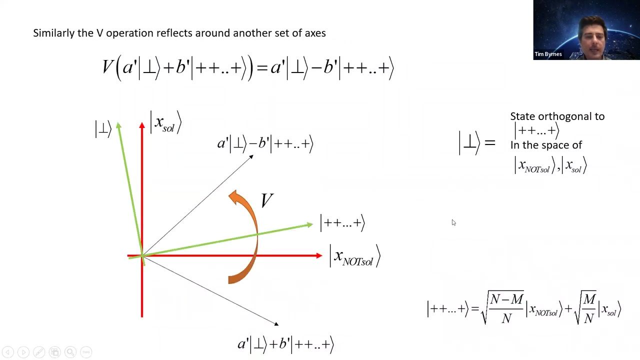 So remember these factors of square root of N minus MN and square root of MN, that those appeared. those appeared, I think, when we first wrote this plus state here. So remember the plus state, we wrote it with these factors here. So actually it's nice to just define our angles. 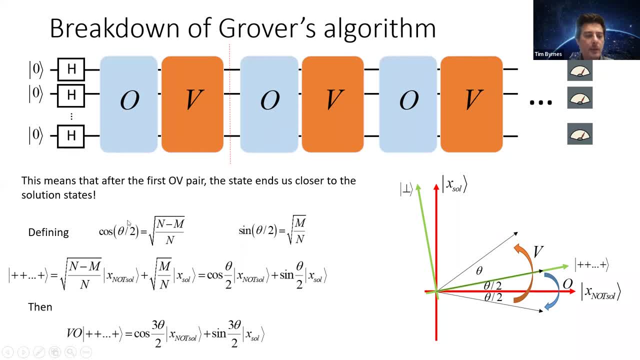 in terms of these values. okay, So we're gonna call this thing cosine theta over two and this thing sine theta over two. Now, of course, sine squared plus cosine squared, it should be equal to one. So if you work that out for these things, 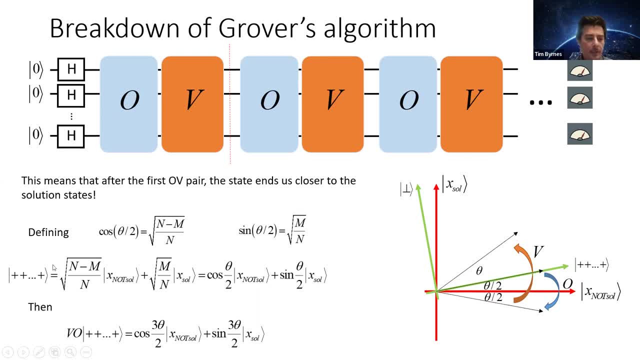 you'll find that it is, in fact, equal to one. So the initial state that we start with. so this is this point in the circuit we can using this definition of theta. we can define it like this: okay, So cosine theta over two and then sine theta over two. 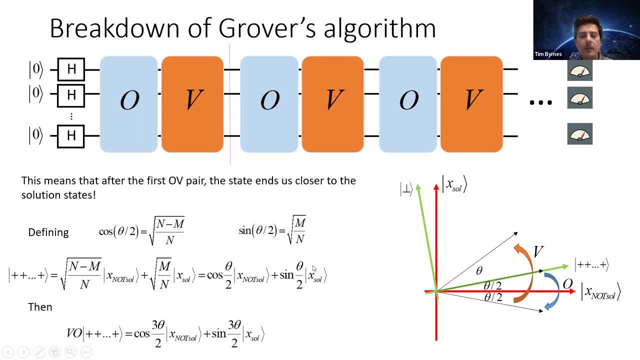 All right and basically using this kind of geometric argument that we're going to call this, you'll see the. So basically you can see that that's the ну state here and, as I sort of kind of argued, the next one is going to be 5 theta over 2.. 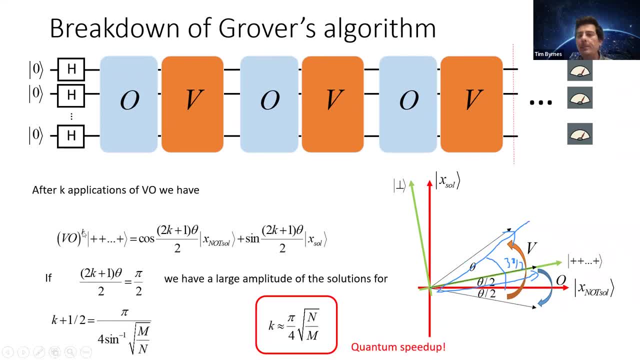 So, in general, after k applications of this VO, you always will have this state like this: So it's cosine 2k, 1 over 2 theta defined on the previous page, And basically what we want to do is, as I said, get this state to be pointing. 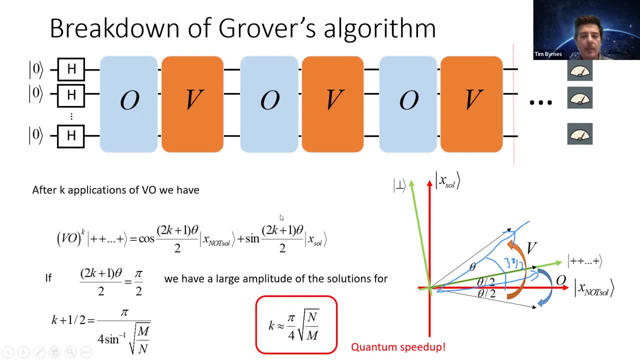 sort of along this vertical direction. So basically what we want is this thing to be 1 and this thing to be 0, because then we'll have the maximum amount that's in the solution states and the minimum amount in the not solution states. So basically we need this thing to be 1,. 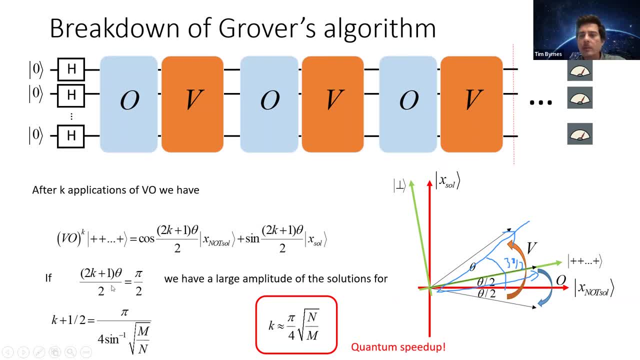 so we can just set this thing to pi over 2, you know, that's when sine is equal to 1.. So 2k plus 1, 0 over 2 is equal to pi over 2.. Rearrange this for k, that's the number of. 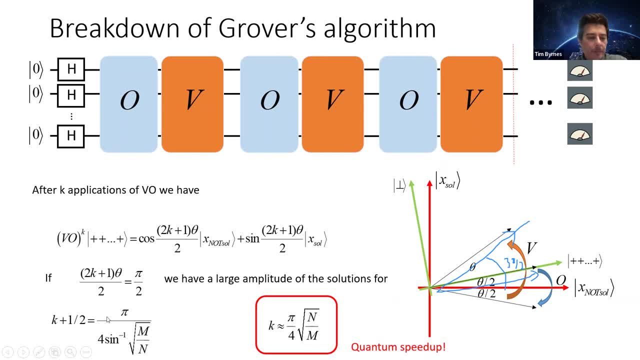 pairs of O that you need to apply. And if you assume that n is quite large, which I guess that's a typical case, then we can figure out that k is something like square root of m. Because you know inverse sine, you can approximate if the argument is small. 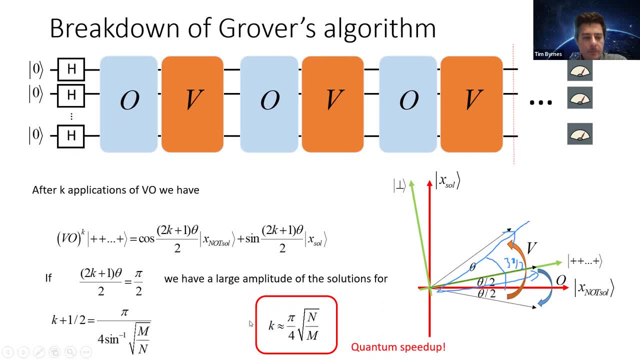 inverse sine is very similar to just a linear function. So k should be equal to pi over 4 times square root of n over m. Now so finally got to the sort of the crunch point, I guess, of that we've figured out how. 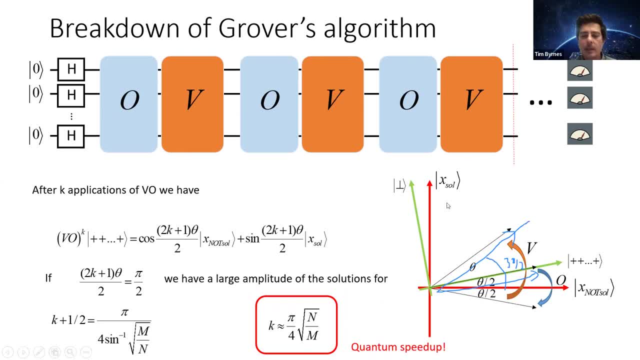 many times we need to apply O to get our result. Now, the key thing is that we've got a square root here, So the number of times that we have to repeat our algorithm is actually square root of n over m. Now let's go back to like basically what. 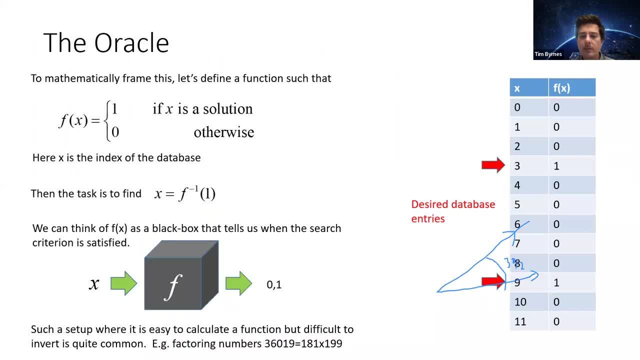 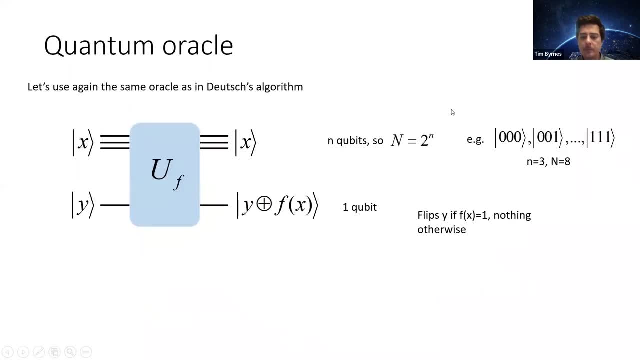 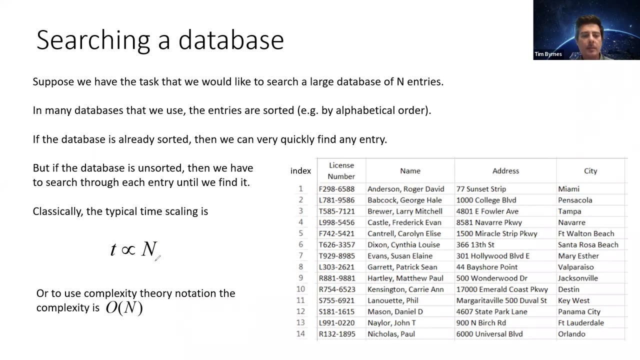 our original problem was. So remember, what we're trying to do here in the first place is we're trying to search for something in the database, And actually maybe what I should have written here is that. you know, I didn't really say how. 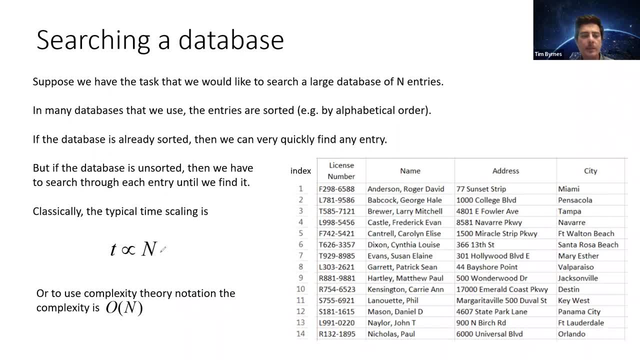 many solutions there were, But obviously if there's like more than one solution, then it's, you know, easy to find. okay, Maybe what I should really say here is, classically, the amount of time that you need should be, should scale something up to the point where 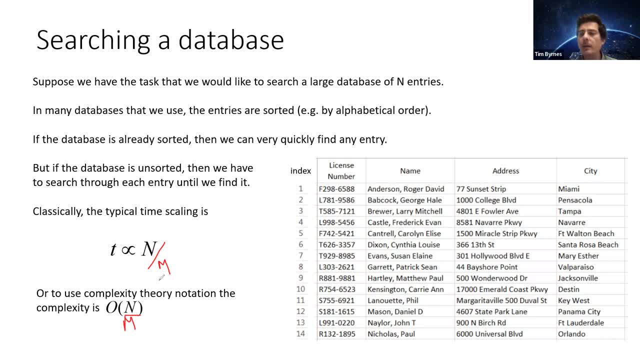 you've got N times this right. Okay, like n divided by m, right because? n because that's the size of the database, right? so if there's 14 entries in your database, then you probably need to look through at least half of it before. 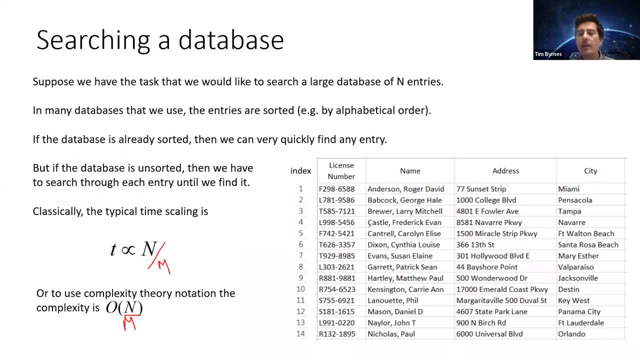 you typically find the one thing that you're looking for, but, of course, if there's more than one answer, you know, like in this case, where I'm looking for license numbers that end in six- well, there's actually two of them right now. if there's two of them, actually, you know, it's twice as likely. 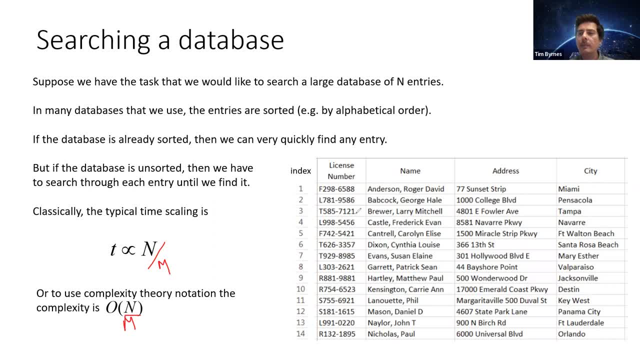 that I find, find it, find a, find it. the correct case, right? so actually you know, the more answers there are, the the easier to find, so the quicker it is. it's defined so classically. the scaling of this search problem is like n over m. now if we compare that to our quantum algorithm. 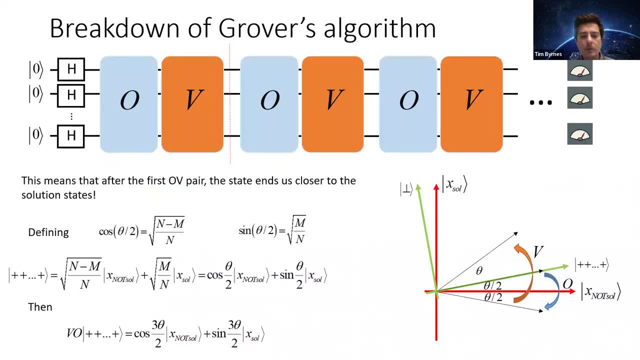 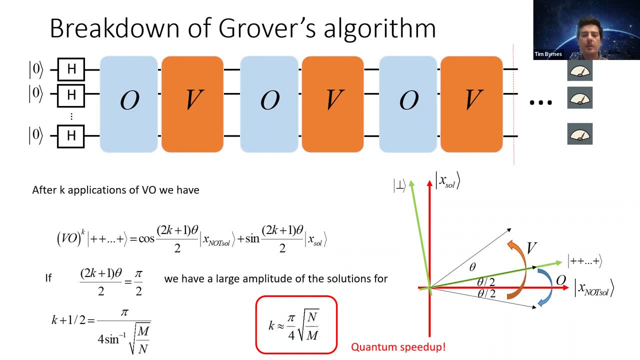 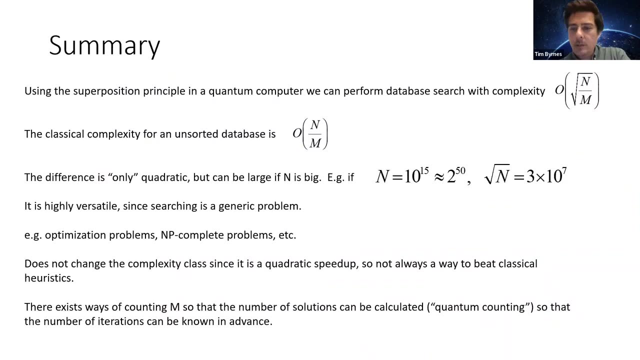 well, so square root of n over m, okay, and pi over four, okay, that's 0.7 or something, so don't worry about it too much. square root of n over n. so this is actually a. this is definitely a quantum speeder because, well, classically, there's really no other way of doing it. 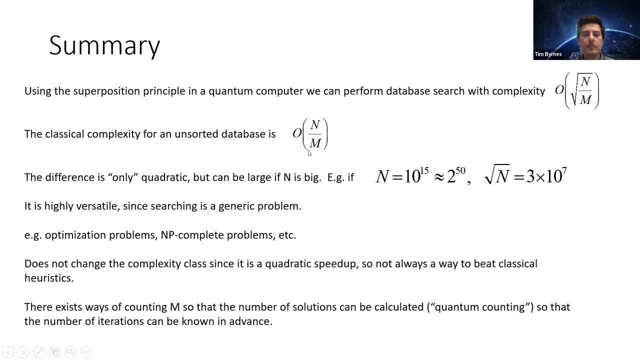 and the only way to do it is to really search through all of them so that scales like n over m, but so quantumly it's square over, you know. so you know it might sound not so impressive like square root factor divided by no square root, but it can be significant because the bigger your n is. 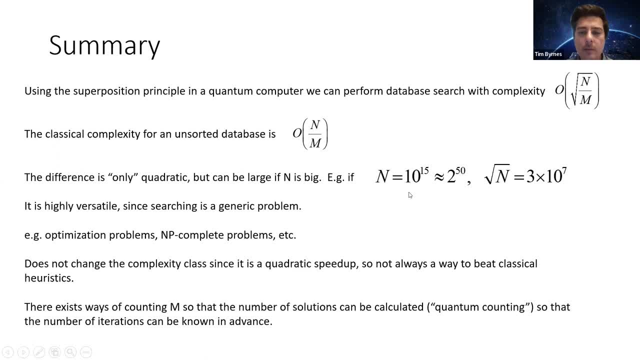 actually the more sort of power that you can sort of see that has. so, for example, if n is like 10 to the 15, you know, I mean this is like you know giga, giga is 10 to the 12, right? so 15 is like tera, right? so you know typical kind of computer sizes of everything. 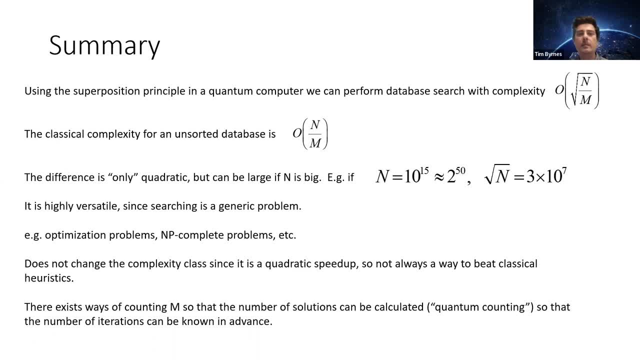 that we deal with these days is, you know, like giga or tera, right. so you know your hard disk might be terabytes. you know processor speed is like gigahertz and so forth. so you know like we live in a world where giga and tera are sort of typical numbers. so that's why. 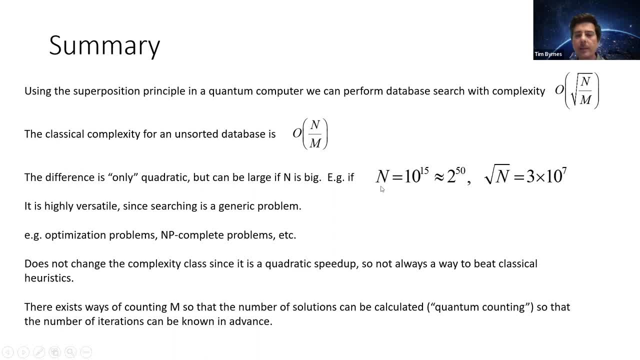 I chose things like tera, so you know that's a fairly big database. I'm searching through it. you know it might take a bit of time. so you know something with 10 to the 15 entries, which is to the power of 50, might be, you know, a realistic kind of problem size. but if it's 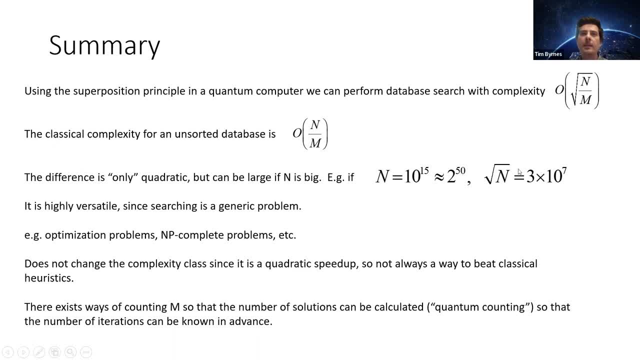 square root of that. that's only 10 to the 7, okay, and 10 to the 7 is, you know just something. it's like mega, or 10 mega, something right, 10 megabytes or something like that. you know, these days, you know, transferring mega something is, you know, pretty, pretty easy. so you know it can. 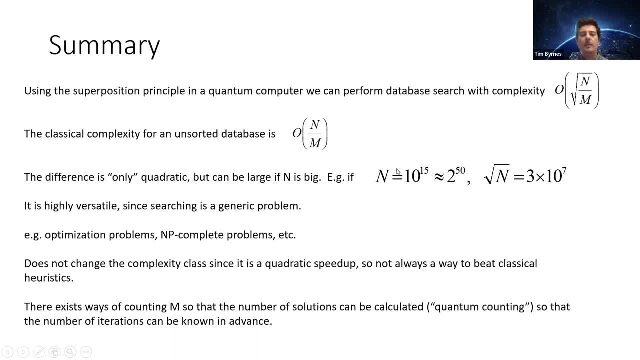 make big difference. obviously, if these numbers are even bigger than then it's at. the speed up factor is kind of bigger. another thing is that it's very versatile. so you know, because searching is such a generic problem, like you search in all kinds of contexts, well, obviously we search stuff on the 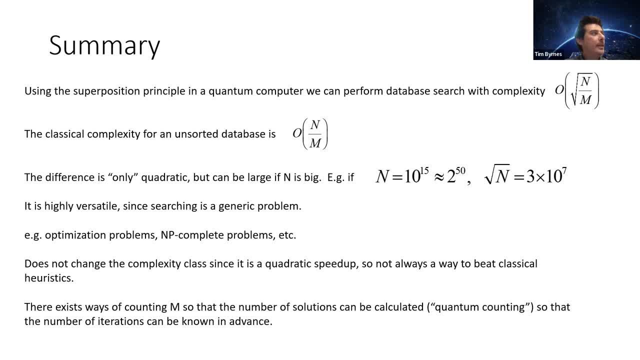 internet, but probably more actually relevant is things like optimization problems. so in all kinds of areas of science, engineering, you often are always wanting to optimize things right. so that's some variables and you want to find like best parameters for it. so you know this is potentially applicable to such situation. so I do mention that. so you know, even though this is very applicable, 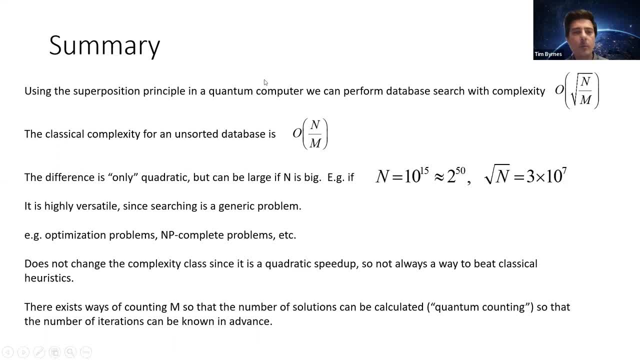 it's not always a clear winner because there's also many good classical kind of heuristic algorithms. so you know, if you say that basically this is going to be faster than you know anything, you know if you built a quantum computer then this would be definitely faster. I think it would be still a case-by-case basis, so I think you couldn't. 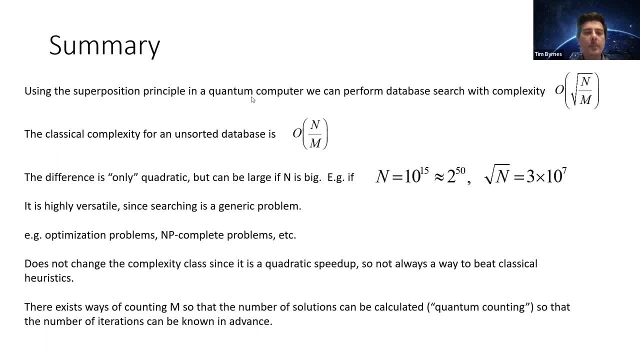 always claim that this is always going to make any kind of computation, like involving optimization, faster, because really depends upon problem, but potentially something you can apply it to a lot of cases and hold on. is this the last slide? guessing? so finally, I think the last thing is maybe a question that you might have had. 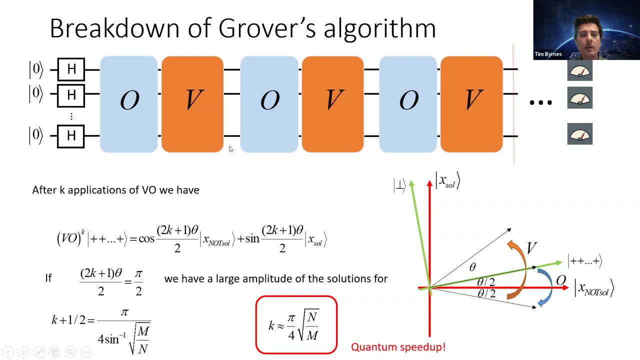 is to say: okay, well, how do I know how many times I'm supposed to apply this obi? because obviously you don't know the solutions you're looking for, the solutions that you know. that's the whole problem. um, how do i know how many times? because because, uh, you know, if you don't know anything about. 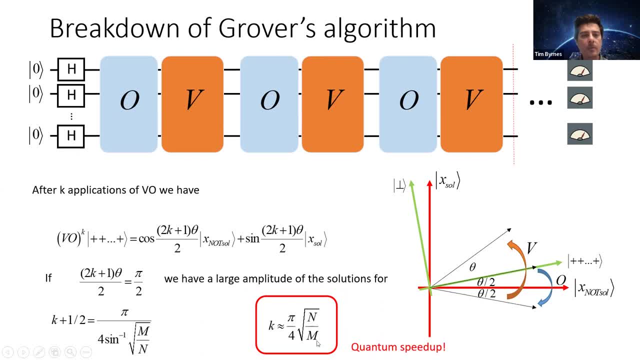 solutions, and you also might not know anything about the number of solutions. you probably know something about the database size, because that's basically related to the number of qubits, but the number of solutions might be actually unknown. so what do you do in that case? well, uh, there's. 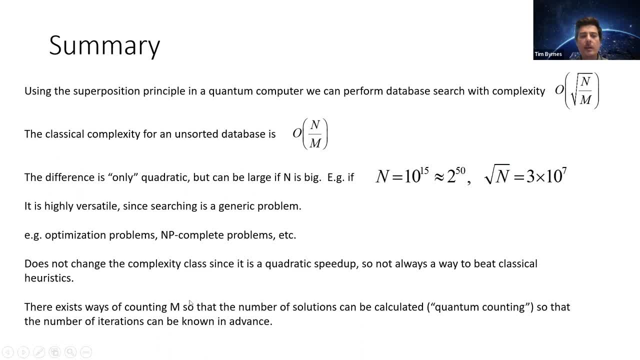 actually some quantum algorithms that can actually uh allow you to estimate m. so, actually, um, this, this can be done- i'm not going to really describe it, but, um, there are certain things called quantum counting, uh, so that you can know what actually m is, and then, in that way you can. 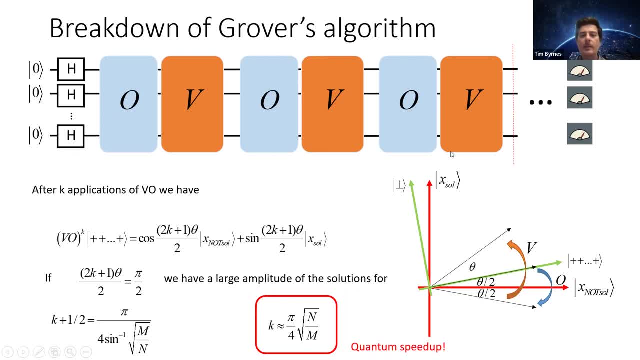 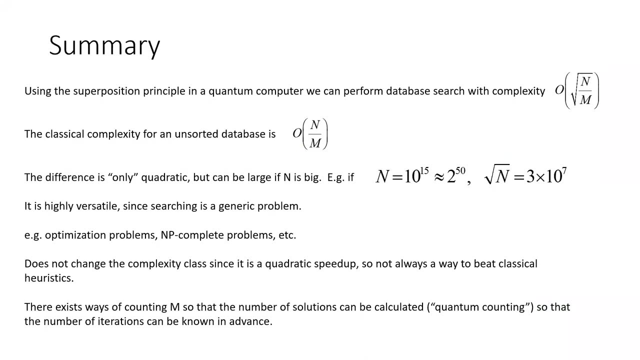 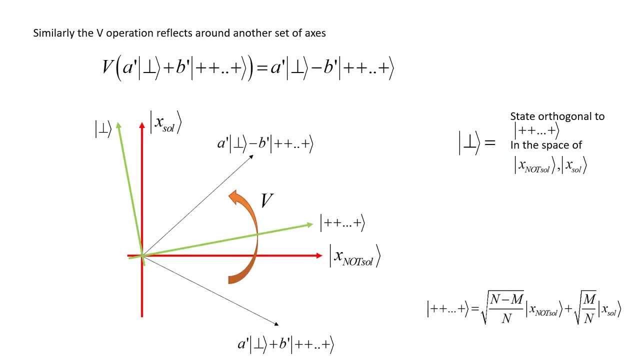 actually figure out, well know in advance how many times you've got to apply this ob sequence. okay, so i think that's that's all um any questions you guys have. i have a question like in in the uh face flip, uh, uh, uh. yeah, when doing face flip it's like 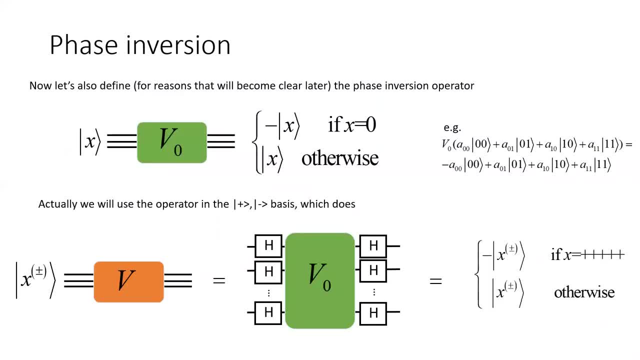 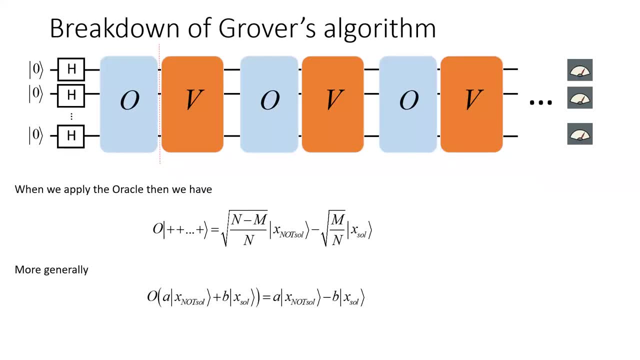 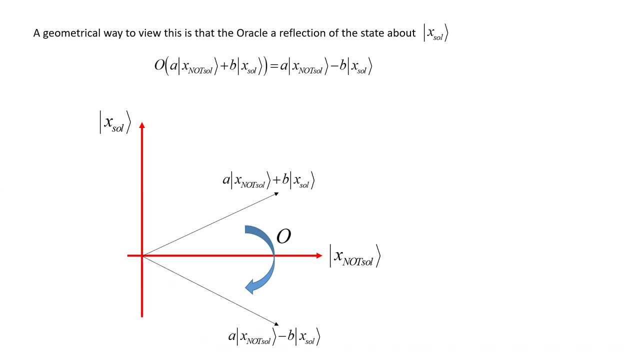 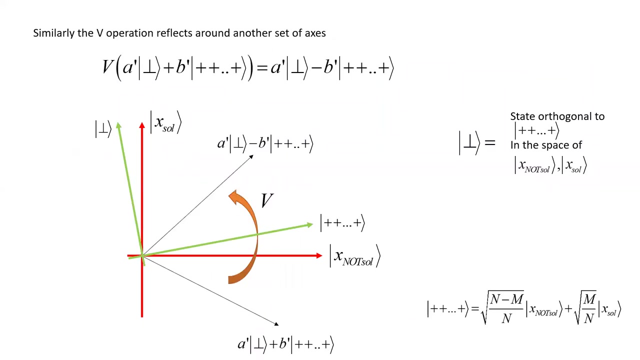 uh, reversing this first step sign. but in the uh, in the graph you've shown, it was like flipping like the um, like flipping the the other, like if you, if you like, do the, do the uh, uh, like the rotation around around the the a plus, plus, plus plus state, and it wasn't like uh, like adding a minus sign in front of the plus. 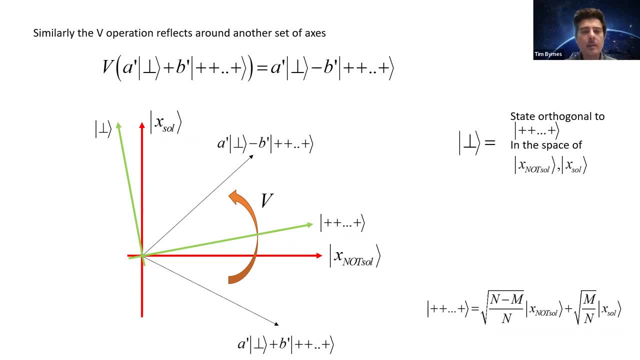 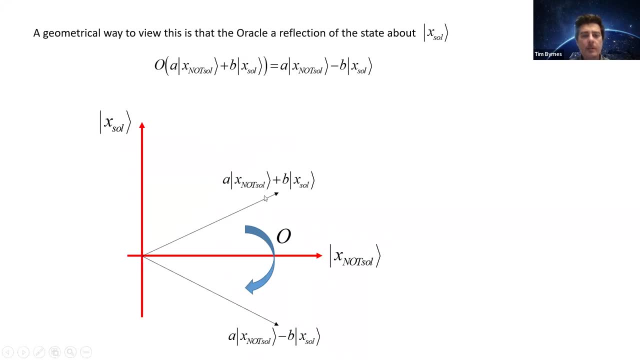 state but yeah, so i think, yeah, maybe, so i think, maybe- let me try to just rephrase the question just to see if i got it right. so, um, i think maybe what you're saying is that. so, according to this, then the axes that you uh rotate around is so, if the oracle applies, a minus sign to the solution. 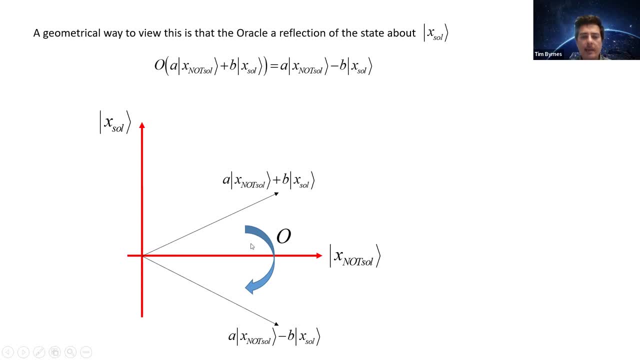 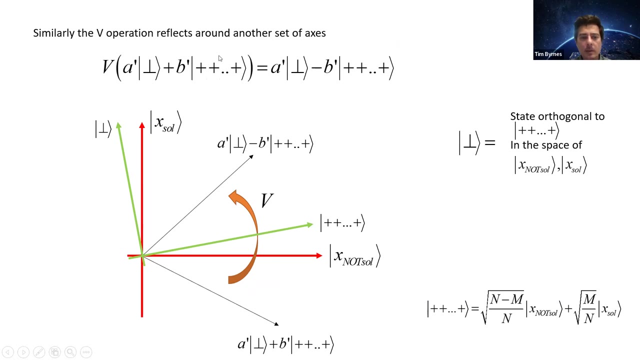 state, then basically the axes that you go around is the, the other one, right, not solution? so by that logic, the b? um, where which applies the uh minus sign to the plus state, should actually rotate around the this perpendicular state and not not the plus state as i drew here. is this your question? yeah, yeah, yeah, i think you're right, but actually in the end, 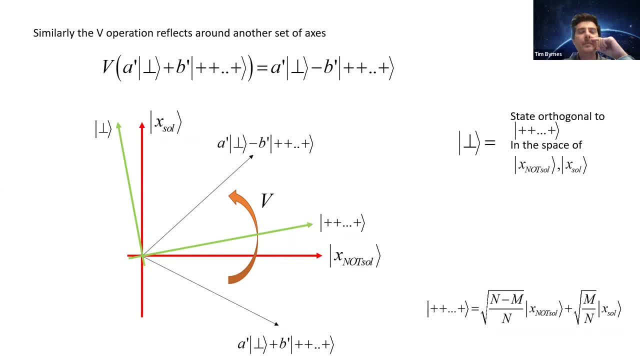 i think it doesn't matter. um, now i uh, okay, the reason why i say i think it doesn't matter is that i could have defined this b state- and probably i should have done that so that it's clearer- so i could have defined this just with the overall minus sign everywhere. okay, so i think i could have defined it, uh, like this: 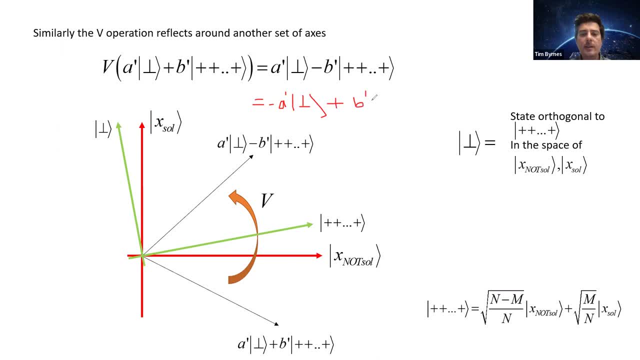 okay, so the the plus sign on the b and then okay, and then a minus sign on the perpendicular, okay, so if i defined it like that, i guess you wouldn't have had any problem, right? um, yeah, but, uh, but, because this one is actually just minus of b, right? and if you think about what? 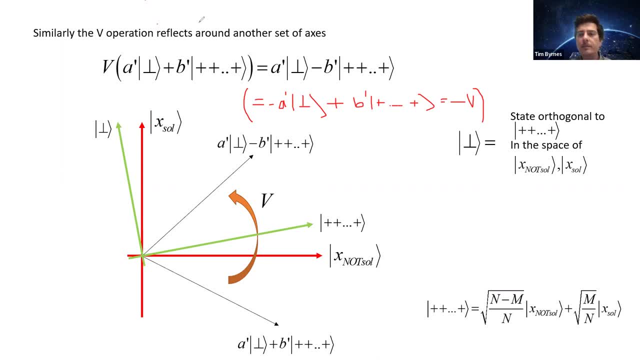 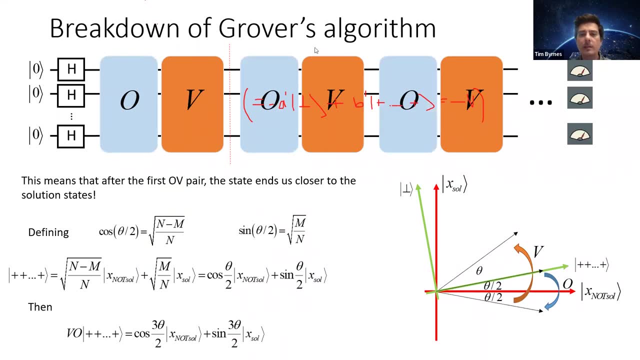 this circuit is going to do, um, basically, if, if i just defined all these instead of v, as i think, if i define as minus v everywhere, basically, this just adds a global phase to everything and i think in eventually, it really doesn't matter. um, so, uh, okay, so that that's why i think it actually shouldn't matter. 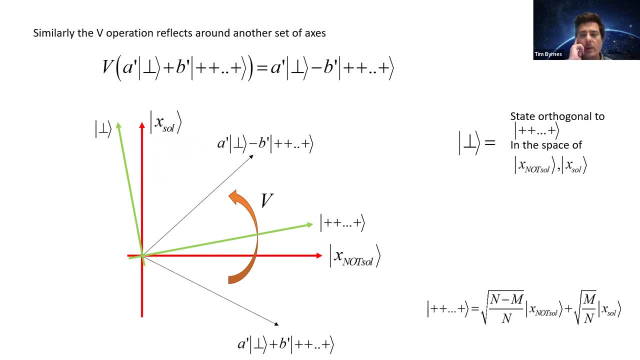 but then geometrically, uh, why would this be actually the same? um, it's kind of a good question, uh, i think i might sit down and think about it, um, so. so yeah, i i can't see geometrically why, uh, but i mean i think it it should be basically the same um. 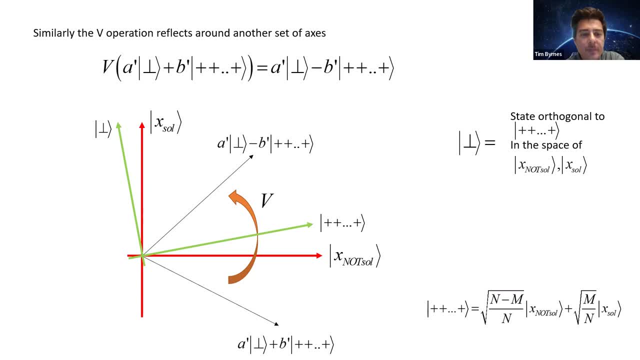 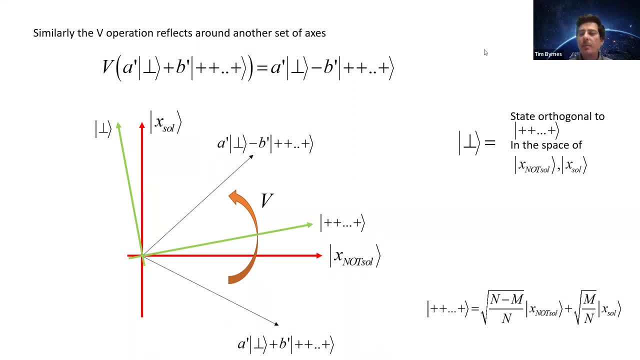 yeah, okay, uh, yeah, so that's a good question. um, probably i should have just defined it the other way and then there will be no confusion. okay, um, but uh, yeah, yeah, i think in this way, like we can always define it as the, as the way we want to like to better show in from actually, yeah, you cannot define it. 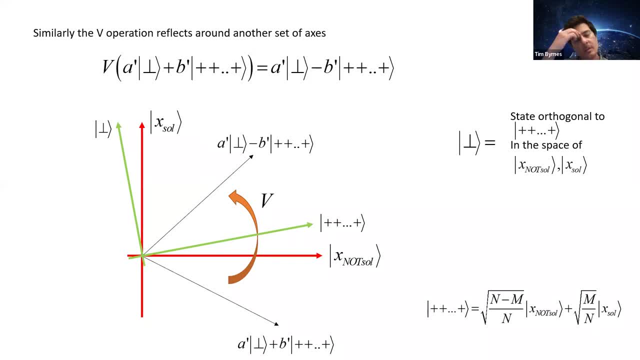 yes, exactly, yeah. so this is a it's like, uh, like, if we start with minus, yeah, we might easily it might mean yes, because then we can use it to count minus, but you know you shape a block. funktioniert it to carry out in terms of the following certain phase time? 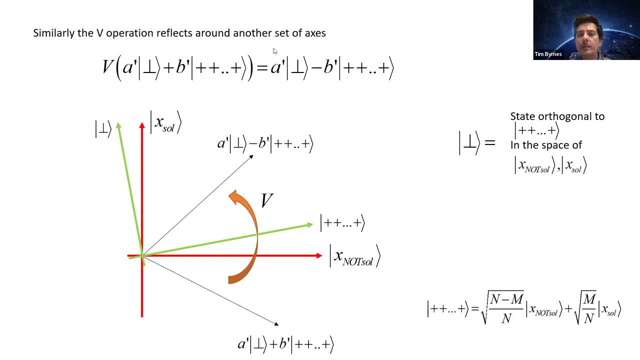 so it would be like komi, where the input value of y equals one times uh, the function- sorry, like the operation byte that you would want to manipulate, right? i can't see my bad way to explain theiminus, right? um, because you, it's a exploit array, so you know, you just. 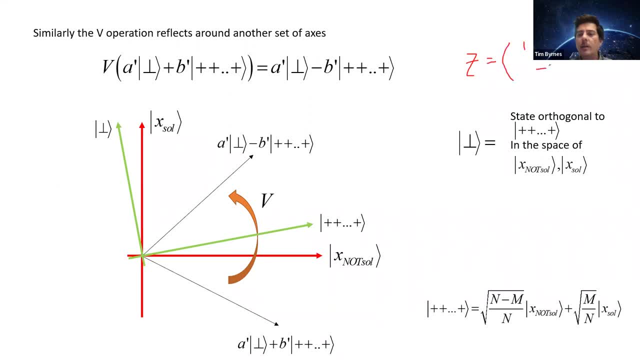 Z operator basically applies one to one side and then zero, sorry, applies a minus one phase to one state and then one phase to the other one. Now, minus Z, of course, just does it the other way around. So minus one one. 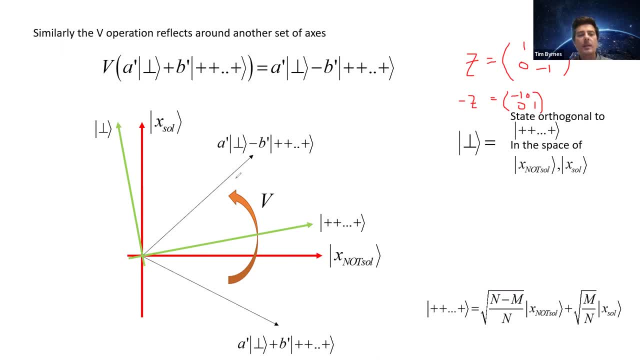 But again, this is just a global phase and what I guess should really matter, I guess should really matter, is only this relative phase that actually they have between them. So yeah, or perhaps even geometrically would this still actually work. So let me just well, I don't wanna say 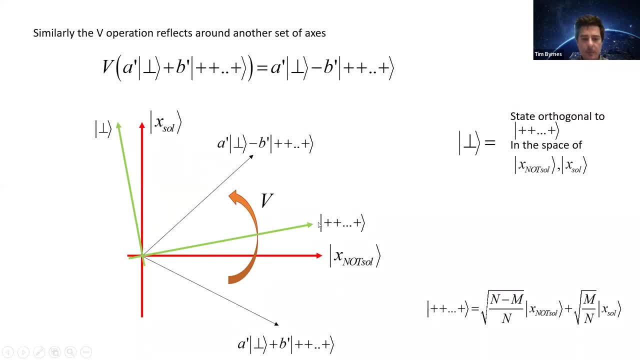 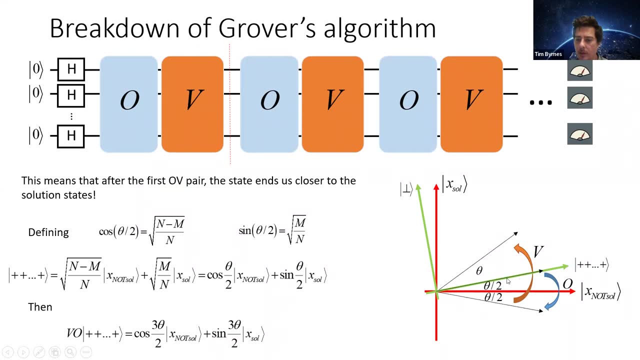 spend too much time doing it. So, for example, over here, suppose that okay, So first step, we rotate around this. not so okay. Then suppose actually, maybe what I, to be perfectly consistent, I should actually reflect around this axis. 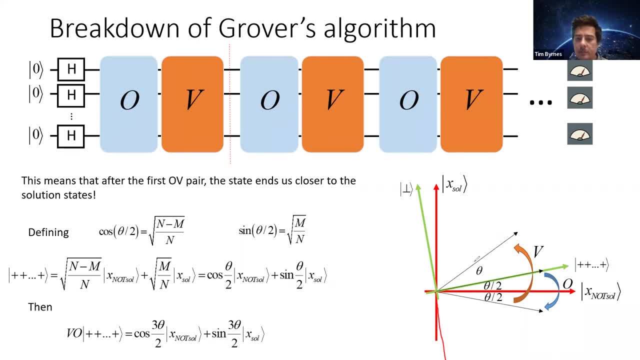 Maybe I'll use green around this axis, Right. Then basically, what will happen is that this vector will end up this way: I think it ends up pointing exactly the opposite direction to the original vector. okay, And then I think, if it points exactly, 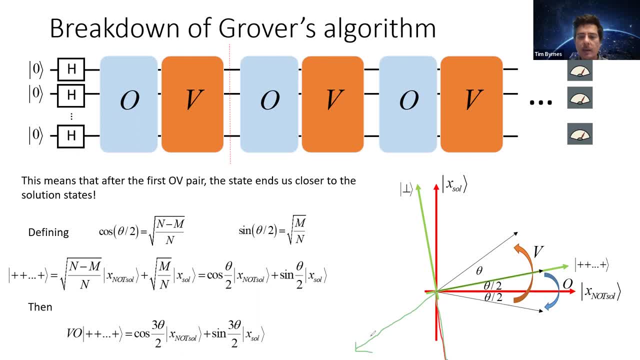 in the opposite direction to the original vector. it is again, just if you think about it. I guess just the only different thing about it is that it's a global phase, and then i think actually there's no, no difference. um, but probably. uh, if you actually did this and then continued. 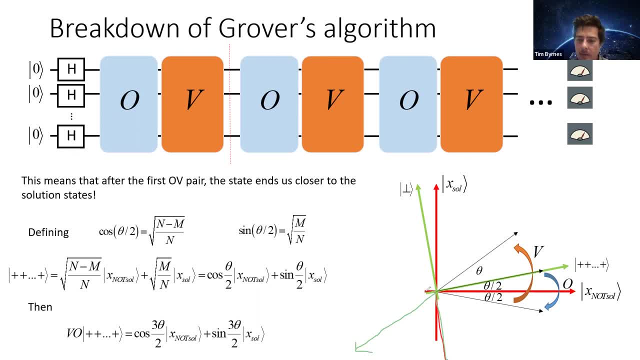 with the sequence where again, all right, now you. so here's. here's what happens after the first step, right, yeah, yeah. and then the second step: now it reflects around this axis, so it ends up here and then, finally, we reflect around this axis, so it goes from here to here and then here. 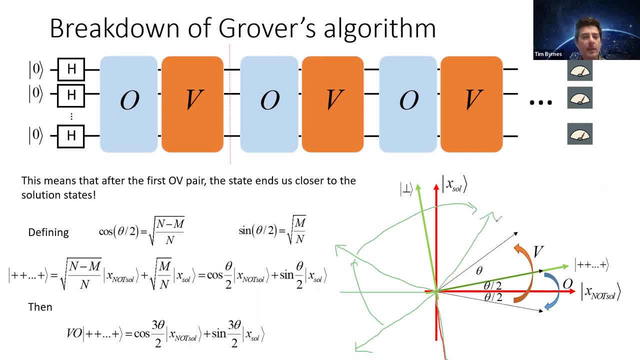 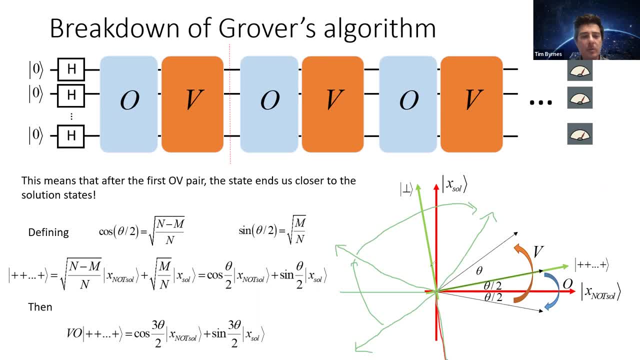 it actually probably doesn't matter which one you actually do um in the picture it looks a little bit different, but then, uh, eventually it will still reach the same um direction. and then, after two, two rounds of ob's, then the minus signs cancel and then there really is no difference. 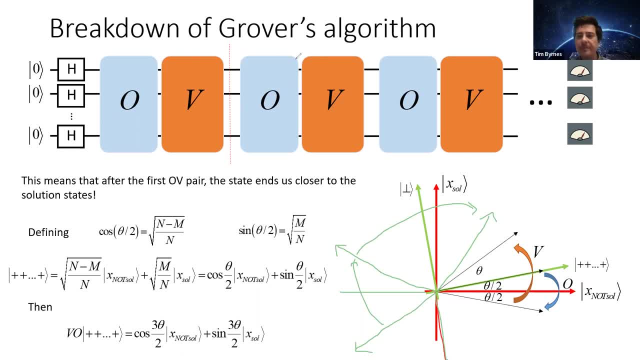 okay, all right. okay, but that's a good question. um, any other questions? okay, oh, it's basically time now, so maybe we'll finish up there. so in the next lecture, do you guys want to do revision? maybe? maybe you probably do yes, yes, okay, all right, so maybe we should. 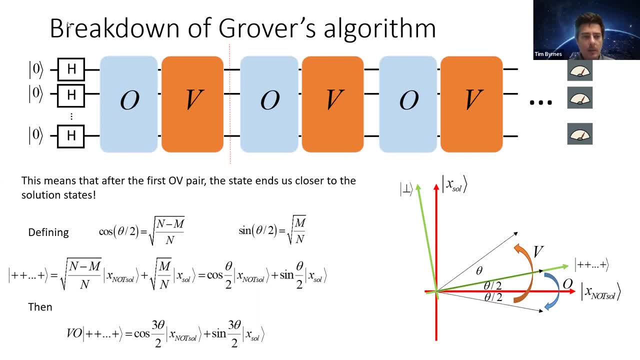 uh, um, you know, basically say that this will be the last lecture in terms of new content, um, and then in the next, on a thursday, we can just, uh, just revise things and just go through any topics that you felt like you want to understand more. so, yeah, maybe you can come prepared with